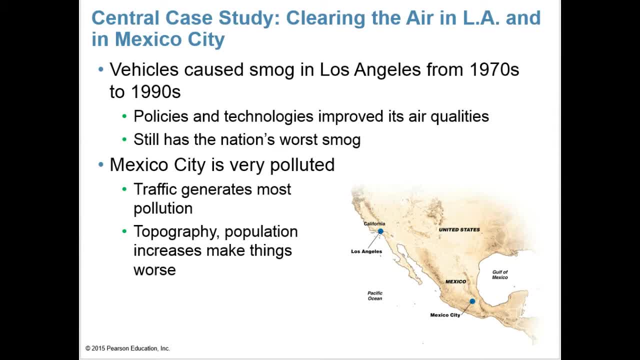 The Sister Cities Program was devised to foster peace and understanding among nations and links hundreds of US cities with foreign counterparts through shared government visits and cultural ties. And one of LA's sister cities is Mexico- Mexico City, which is the capital of Mexico, and one thing those two cities share is smog. 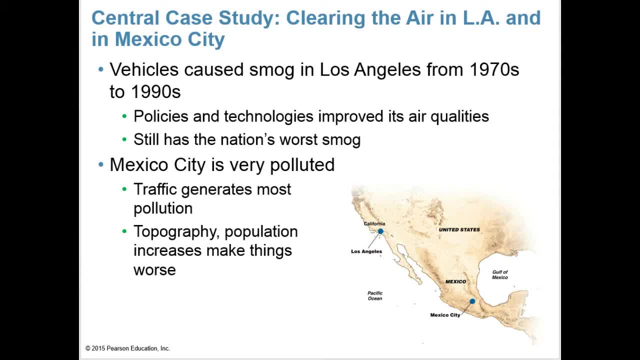 And not long ago, Mexico City suffered the most polluted air in the world, And that's also because of a lot of traffic and automobile exhaust. In fact, there were times where teachers would even keep their students inside, not letting them go out for recess. 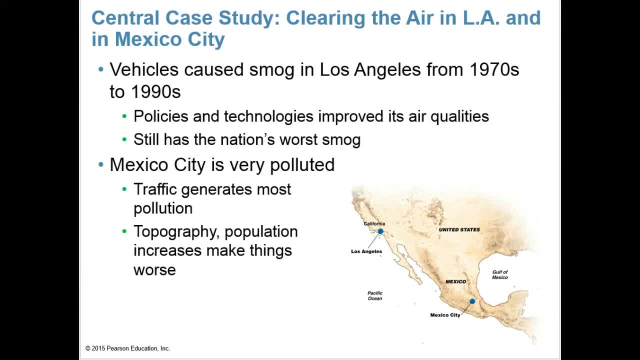 And outdoor sporting events would be canceled, And even children would draw pictures and use brown crayons to color their sky instead of blue. Each year, thousands of deaths and tens of thousands of hospital visits were blamed on the pollution in Mexico City. Like LA, Mexico City is surrounded by mountains, which allows thermal inversions to trap pollutants over the cities. 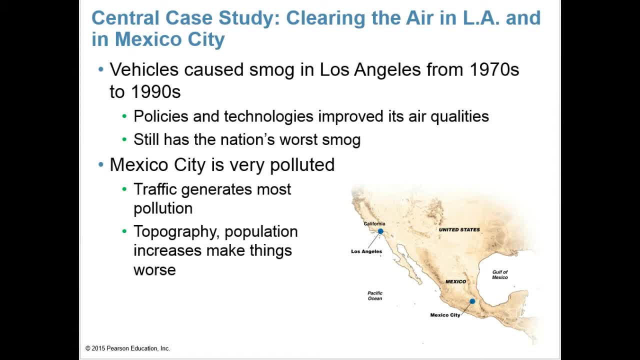 Plus, at its high altitude the air is polluted altitude Solar radiation is very intense in Mexico City and it also helps to trap smog by the interaction of pollutants with sunlight. So people have kind of laughed and said that Mexico City is like a casserole dish with a lid on top. 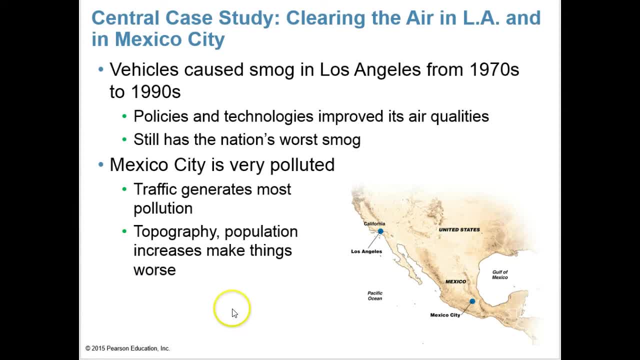 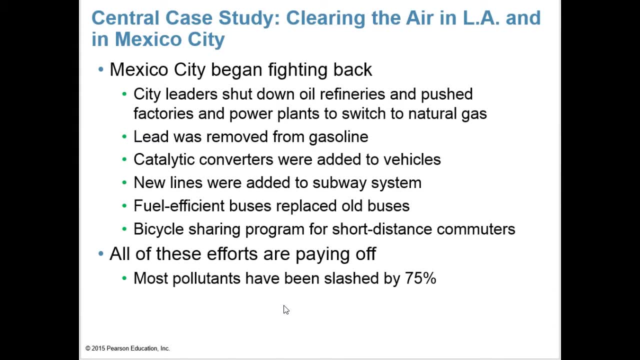 trapping all of the pollutants and smog within. But Mexico City has been fighting back. Efforts began in the 1990s, when city leaders shut down an oil refinery and pushed factories and power plants to shift to cleaner burning natural gas. Lead was removed from gasoline and the sulfur content of diesel fuel was reduced, and 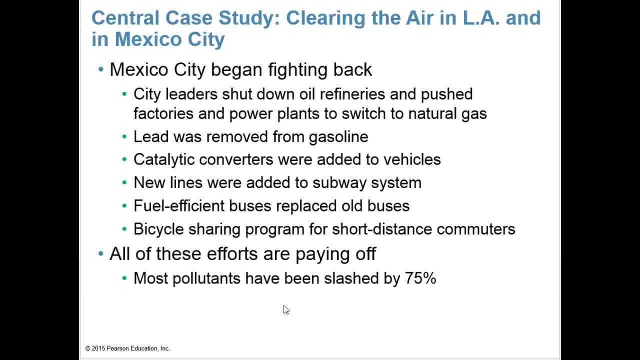 pollution control technologies like catalytic converters were phased in for new vehicles, Levels of many pollutants fell, but as the city grew, smog from the automobile traffic still persisted and in response, city officials stepped up vehicle emission testing and upgraded their taxis and city vehicles to cleaner models And to monitor air quality. 34. 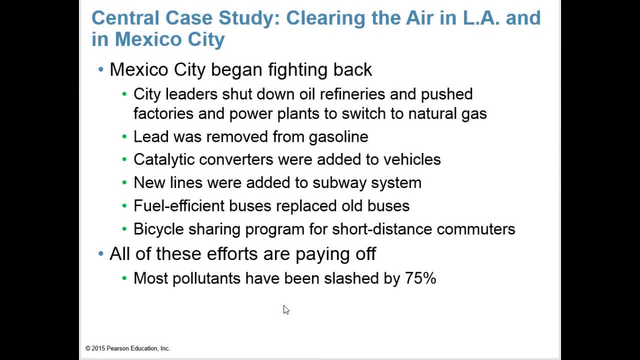 sampling stations were set up across the city, sending real-time data to their engineers. New lines have been added to their subway system, and they've gotten rid of 800 old buses and replaced them with newer, fuel efficient ones that over 450,000 people use today. In fact, they've thought that they've cut out carbon dioxide. 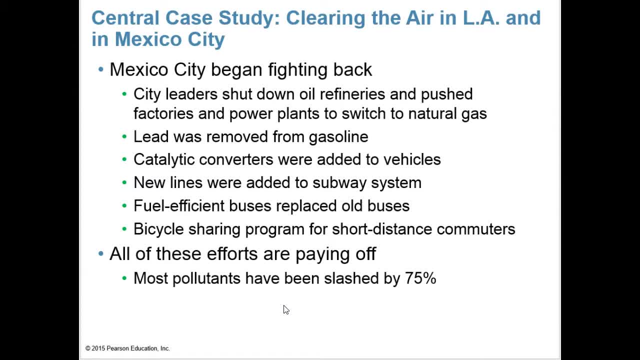 emissions by an estimated 80,000 tons per year. They've introduced programs like bicycle sharing and even car sharing and carpooling programs. Mexico City is following in the footsteps of Los Angeles, and both are making steady progress toward cleaner air, But there's 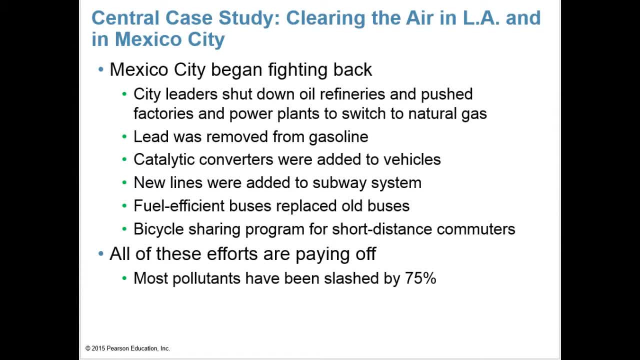 still a lot of hurdles and challenges that still remain as population increases and highways increase, which they fear might make people want to drive more. There are other cities that are considered sister cities to Mexico City in LA. they include Athens, Greece, Jakarta, Indonesia, Mumbai, India and others. 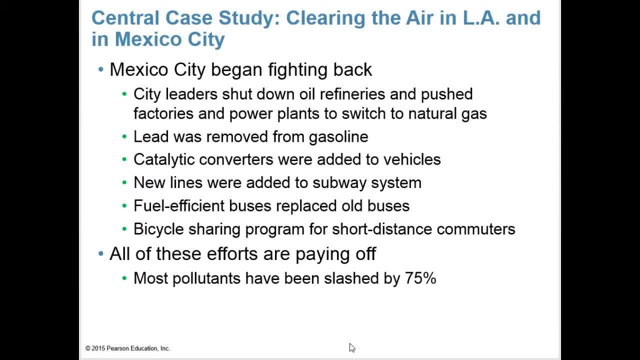 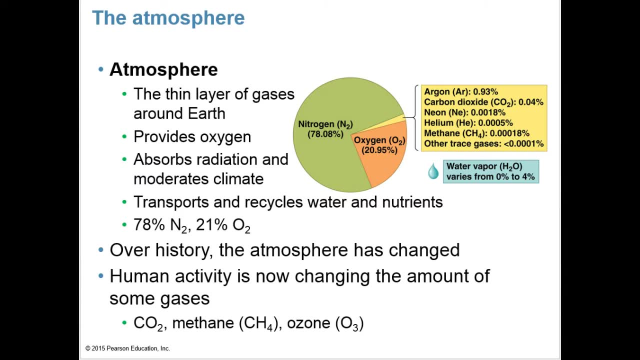 And as we learn about Earth's atmosphere, we'll think about how to reduce the pollutants that we release into it. The atmosphere is the layer of gases that envelops our planet. It moderates our climate, provides oxygen. it shields us from meteors and from hazardous 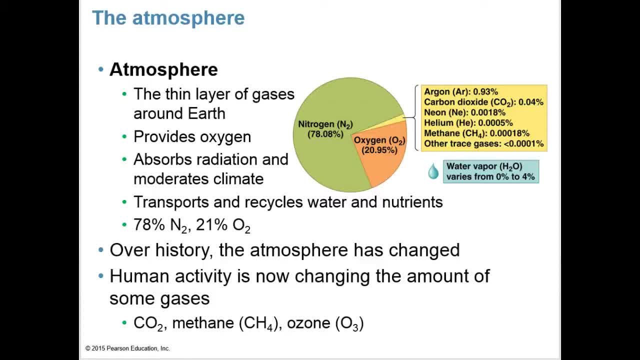 solar radiation and transports, and recycles water and nutrients. It consists of 78% nitrogen, known as N2,, and 21% oxygen, also known as O2.. There's other elements in our atmosphere as well. They include 1% oxygen. 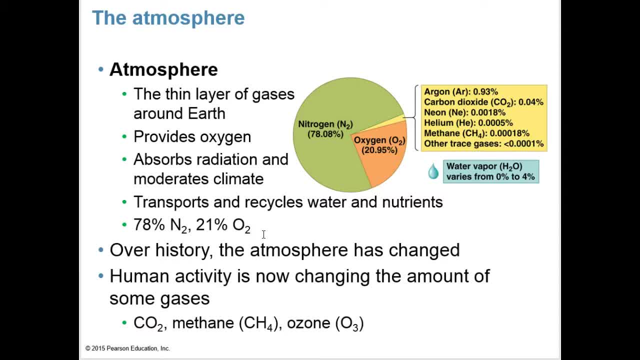 They include 1% oxygen. They include 1% oxygen. They include 1% argon and even water vapor. that varies with time, from day to day, from 0 to 4%. We can see that through Earth's time, the constituents of the atmosphere have changed. 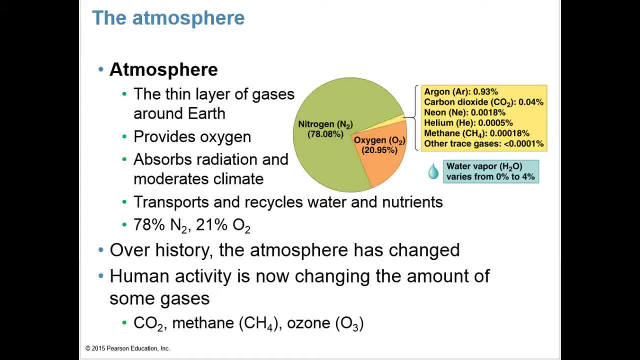 We can tell by looking at rocks and by looking at ice cores in the Arctic. Over human history, we've been monitoring the changes in especially carbon dioxide and methane, known as CH4. And ozone, known as O3.. The Earth's atmosphere is layered. 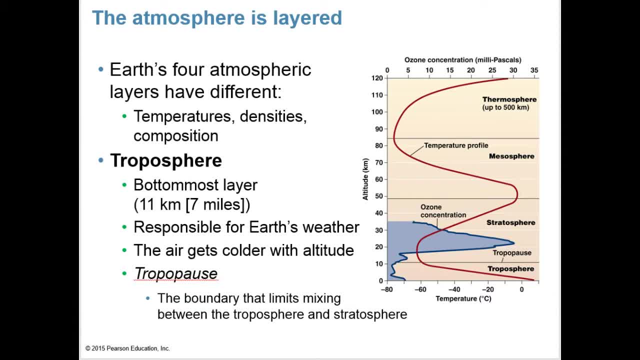 Air pressure and the density of molecules decrease exponentially as altitude increases, but temperature varies in a more complex way, allowing us to identify several layers that have different temperatures, different densities and different composition, And there's four of them. First of all, there's the troposphere. 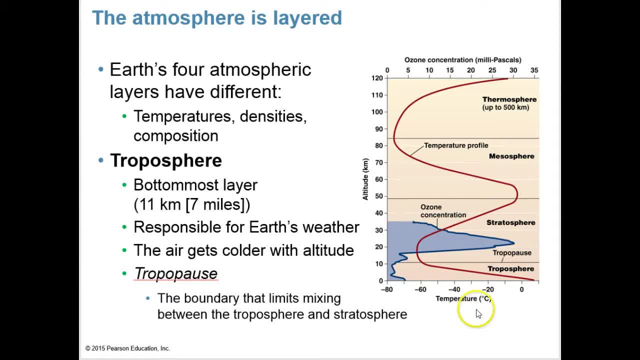 And we can see with the chart here over to the right where that would be located. on the bottom It's seven miles and it's responsible for our Earth's weather. The air gets colder with altitude as you go up. There's also what's called the tropopause. 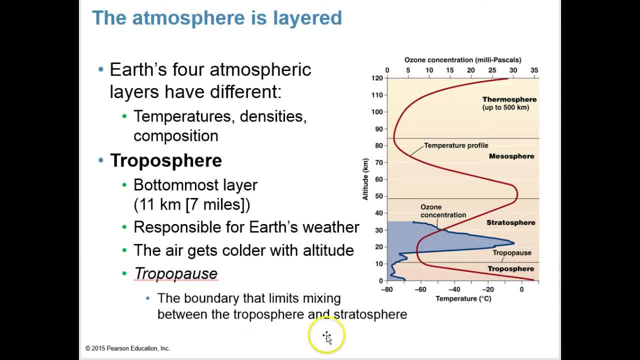 It's the boundary that limits mixing between the troposphere and the next layer, called the stratosphere. Relative to the other layers, the troposphere is actually pretty thin, but it contains three quarters of the atmosphere's mass. The reason is that gravity pulls mass downward, making the air denser near Earth's surface. 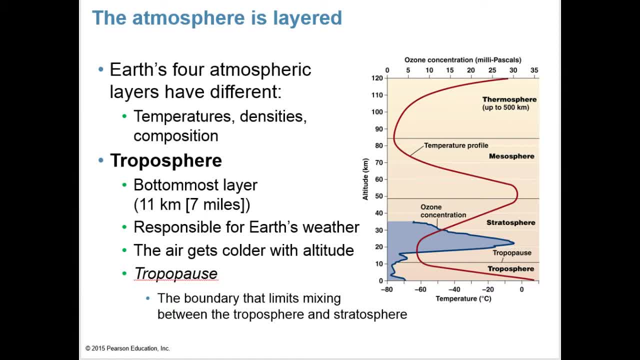 And so tropospheric air gets colder, with altitude dropping to roughly negative 62 degrees Fahrenheit at the top of the troposphere. At that point then, finally, temperatures stabilize, Marking that boundary called the tropopause, And it acts like a little cap limiting mixture between the troposphere atmospheric layer. 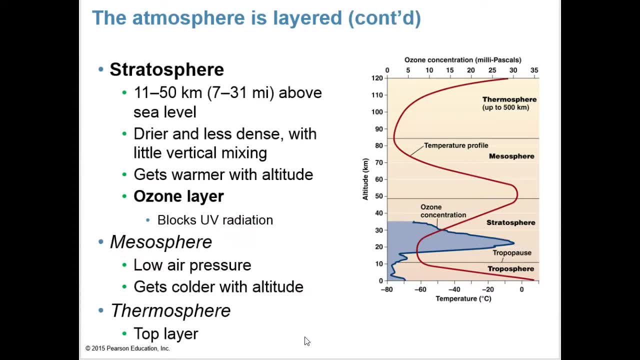 to the stratosphere layer above it. The stratosphere layer, then, which is above the tropopause of the troposphere, is the next layer. It's about 7 to 31 miles above sea level. It has drier and less dense air. 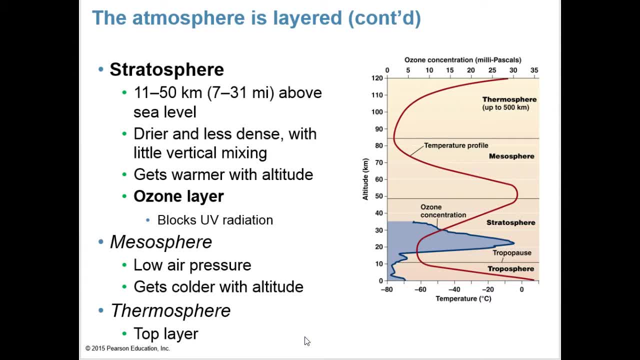 With little vertical mixing, And this one actually gets warmer with altitude. This is also the layer that has what's called our famous ozone layer, And the ozone layer is so important to Earth and us because it blocks UV radiation. UV light can damage living tissues and can create genetic mutations in our DNA. 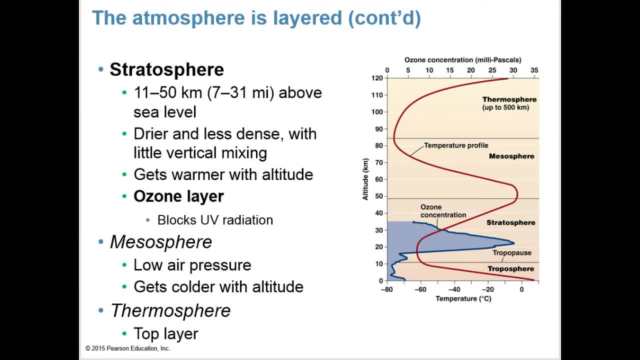 And life has evolved to rely on our protective ozone layer, That's within the stratosphere. Above the stratosphere lies the mesosphere, where temperatures decrease with altitude and where incoming meteors burn up. Above that is the thermosphere that extends to roughly 500 kilometers or 300 miles. 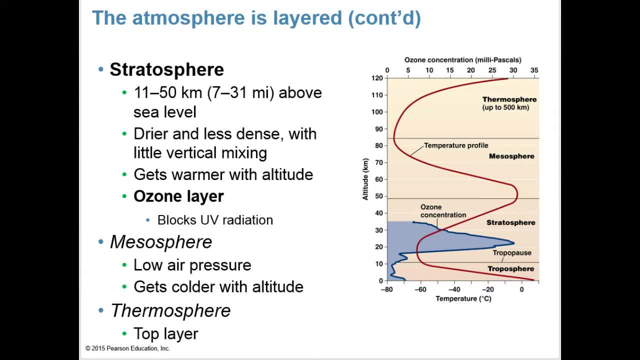 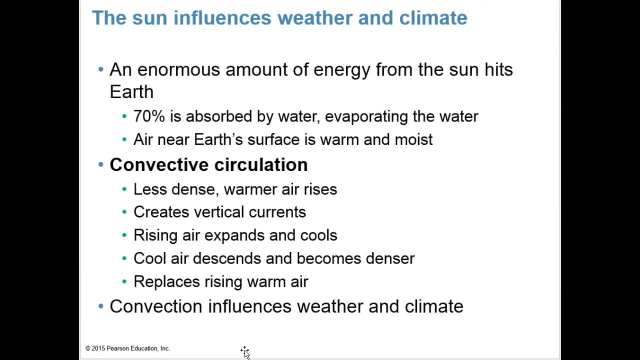 And still higher. yet the atmosphere merges into space in a region called the exosphere. The Sun influences weather and climate. Enormous amount of energy from the Sun hits the Earth and 70% of this is absorbed by water and evaporates the water. 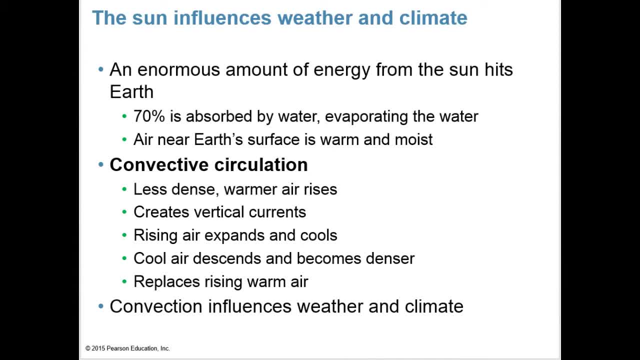 Air near the Earth's surface is warm and moist, then This is because land and surface water absorb Sun's energy and then emits it as thermo-infrared radiation. 3. Diff set into motion a process called convective circulation, and this is how it works. 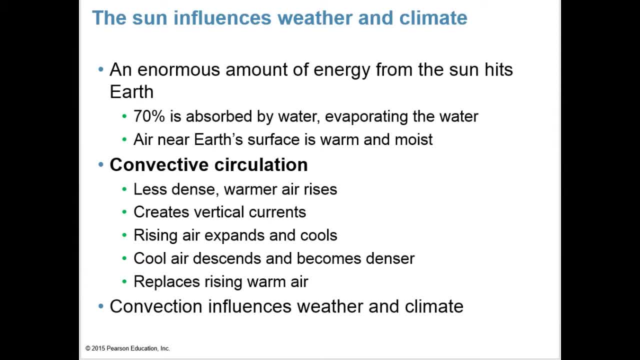 Warm air is less dense, naturally, and it rises and creates vertical currents. As the air rises into regions of lesser atmospheric pressure, it expands and cools, causing moisture to condense and fall as rain. As the air cools, it descends and becomes denser, replacing warm air that's rising. 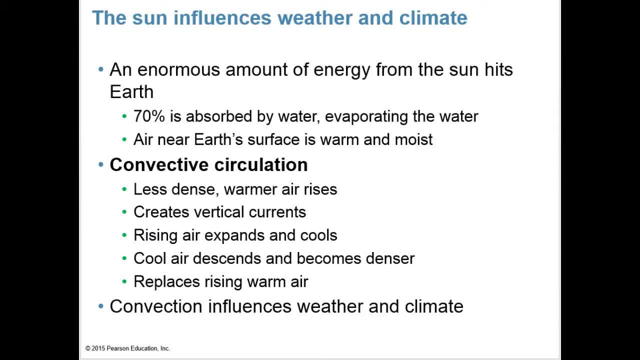 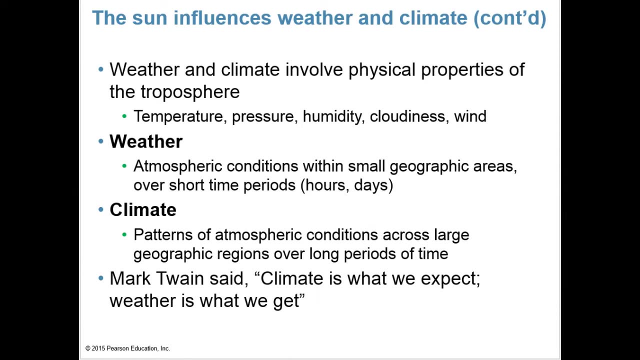 The descending air picks up heat again and moisture near the ground level and prepares to rise yet once again, continuing the process. Convective circulation influences both our weather and our climate. Weather and climate each involve physical properties of the troposphere, and these include temperature. 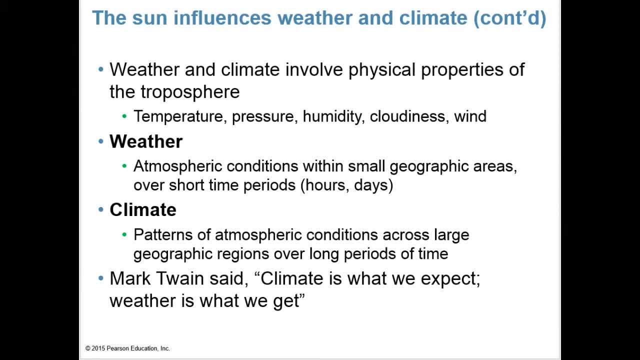 Pressure, humidity, cloudiness and wind. So we say weather is the specifics about the atmospheric conditions within small geographic areas over short amounts of time, such as within hours and days. Climate, then, is more of a pattern over a longer range of time, including decades, years, centuries. 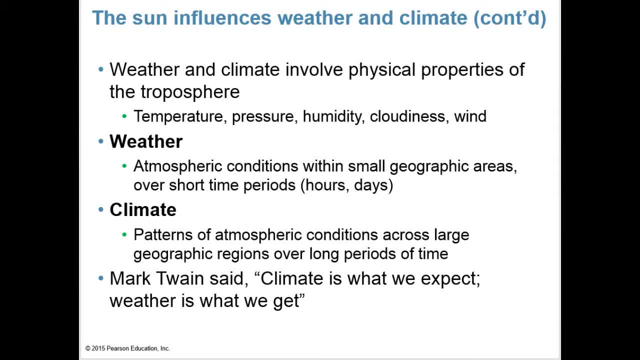 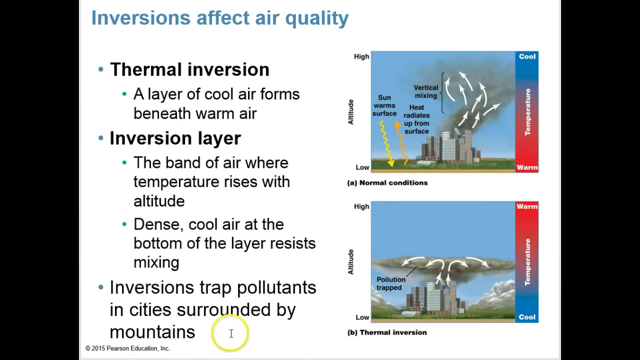 or millennia Famous author Mark Twain. For example, Los Angeles has a climate characterized by warm, dry summers and mild, rainy winters, but yet on some autumn days, dry Santa Ana winds blow in from the desert and bring extremely hot weather. 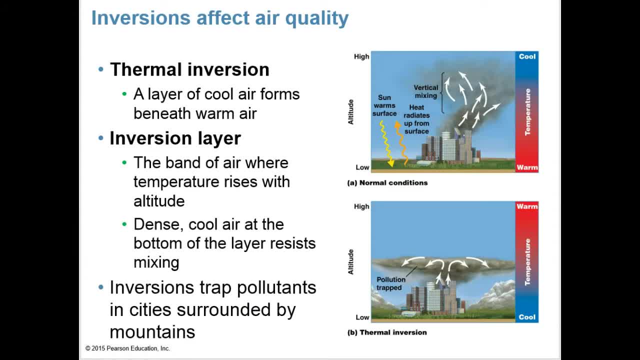 Under most conditions, air in the troposphere becomes cooler as altitude increases, as well as temperature increases. As a result, the air in the troposphere becomes cooler as altitude increases. In addition, there is an生ye change in temperature. A cold air can form beneath a layer of warmer air. 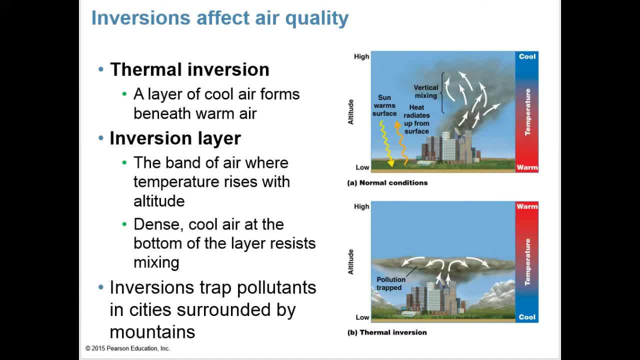 In this case, it is a temperature inversion or a thermal inversion. The band of air in which the temperature rises with altitude is called an inversion layer. This is because the normal direction of the atmosphere changes according to the temperature change. In contrast, in this case, the air in the troposphere is typically warmer. 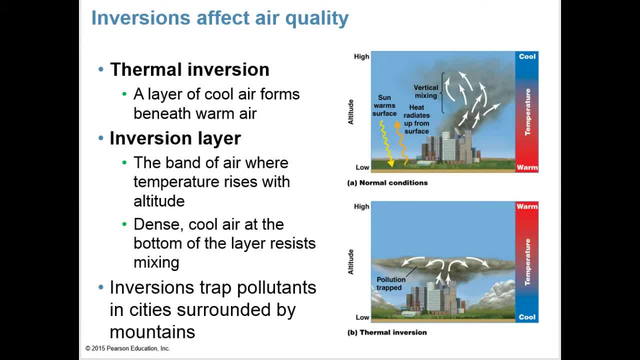 We can see the temperature change in the troposphere. In this case, the air in the troposphere is changing rapidly and indeed the air in the troposphere is here and there and the thermal inversion happens. In other words, temperature turns to be an inversion force. 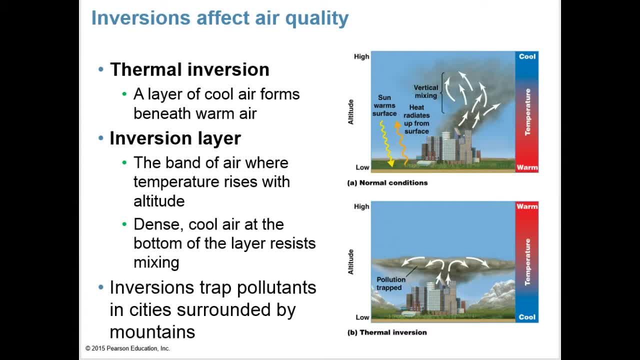 When we resume the thermal inversion, the temperature can continue to improve in order to gain the same level of temperature loss, and it will continue to improve eventually, over time. We can also call this an inversion layer, temperature inversion or a thermal inversion: The band of air in which the 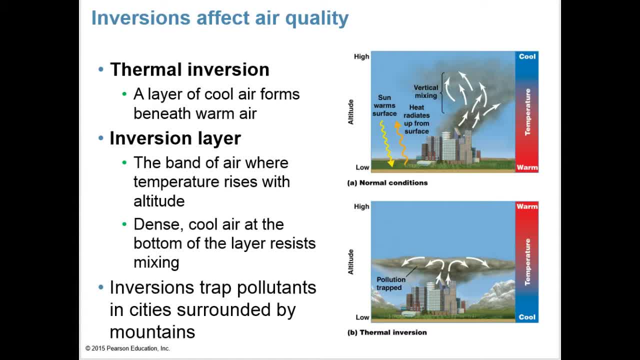 temperature rises with altitude is called an inversion layer. This is because the normal direction of temperature has changed or is inverted. The cooler air at the bottom of the inversion layer is denser than the warmer air above, so it resists the vertical mixing and remains stable. 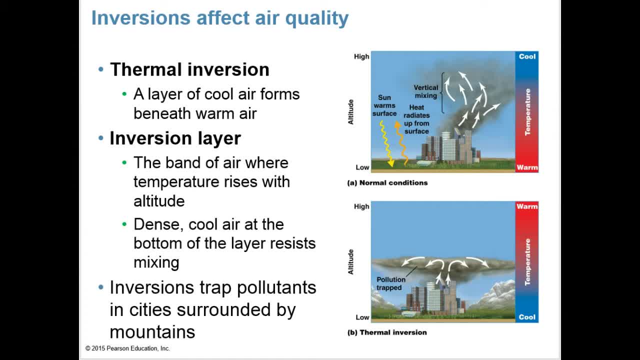 Thermal inversions can occur in a number of different ways, sometimes involving cool air at ground level and sometimes involving an inversion layer higher above the ground. One common type of inversion is shown here in the diagram to the right in the B picture here under thermal inversion. 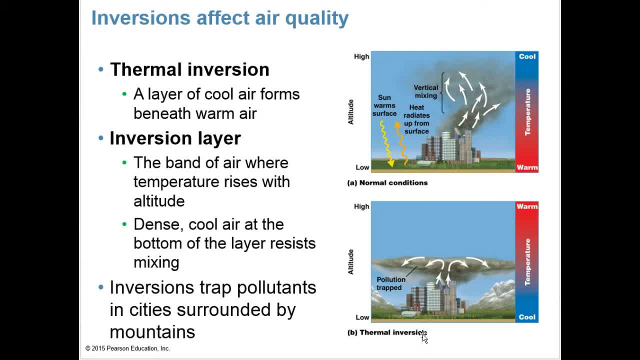 In the diagram to the right in the B picture here under thermal inversion. In the diagram to the right in the B picture, here under thermal inversion. this sometimes occurs in mountain valleys where slopes block morning light and that keeps ground level air within the valley shaded and cool down here. 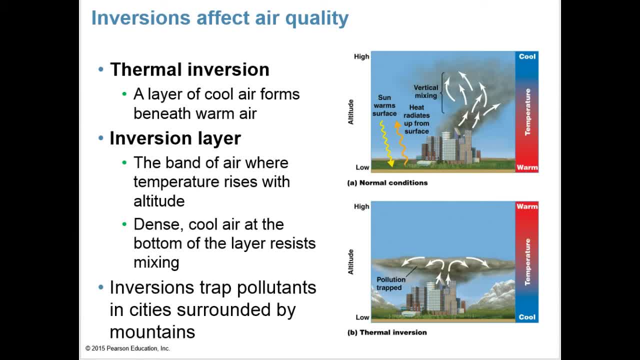 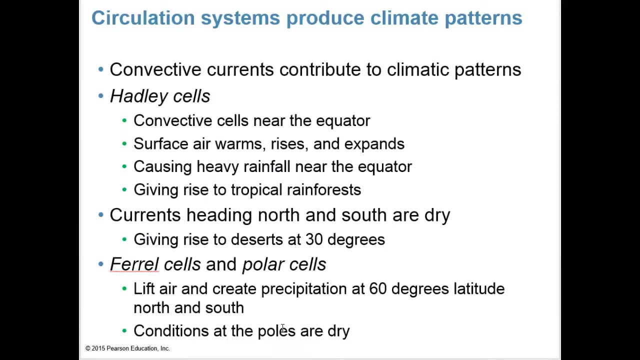 Vertical mixing allows pollutants in the air to be carried upward and diluted, but thermal inversions trap the pollutants near the ground. This is what's happening in places like Los Angeles and Mexico City. At large geographic scales, convective air currents contribute to broad climate patterns. 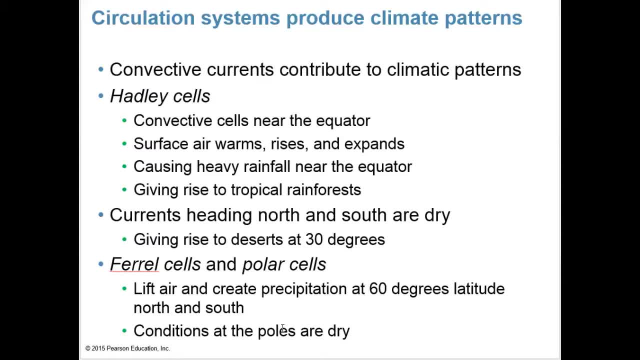 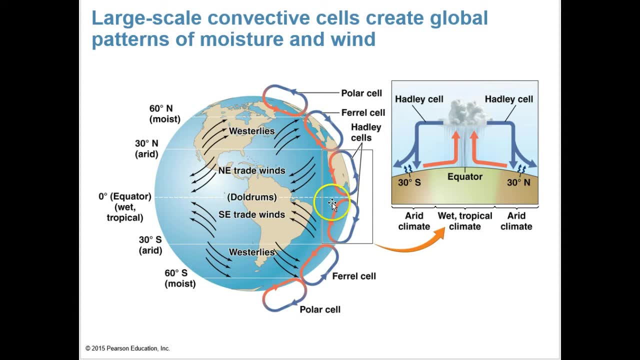 Near the equator, solar radiation sets in motion a pair of convective cells known as Hadley cells. I'm going to switch the slide pictures down to this one here so we can get a look at a diagram of that. Here's the Hadley cells. Here's where the sunlight would be the most intense and 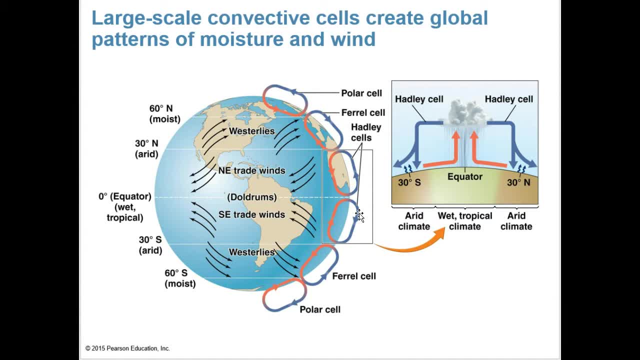 where it would warm the surface air the most. That surface air would then rise and expand, and as it does so, it releases moisture, producing heavy rainfall that gives rise to the tropical rainforests in these areas. But after releasing much of its moisture, the air diverges and 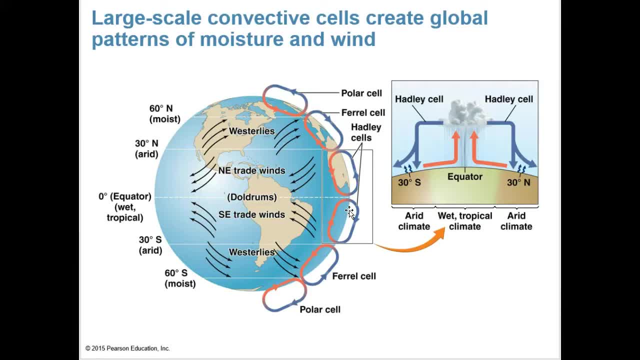 moves in currents heading north and south. The air in these currents cools and then descends at about 30 degrees latitude, north and south, And because the descending air is now dry, the areas around the 30 degrees latitude mark are quite arid or dry, giving rise to deserts. 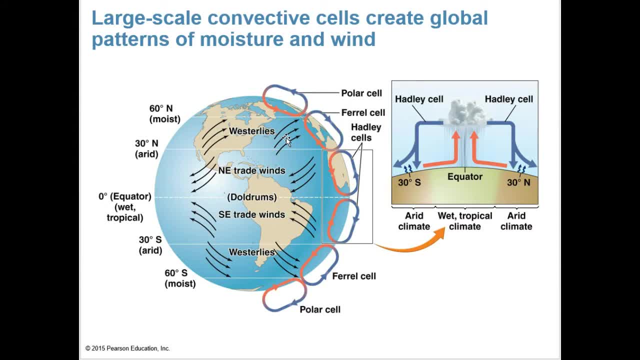 in those areas. Two further pairs of convective cells called ferrule cells, shown in the diagram here in the north and here in the south, and polar cells, again north and south, lift air and create precipitation around 60 degrees latitude and cause air to. 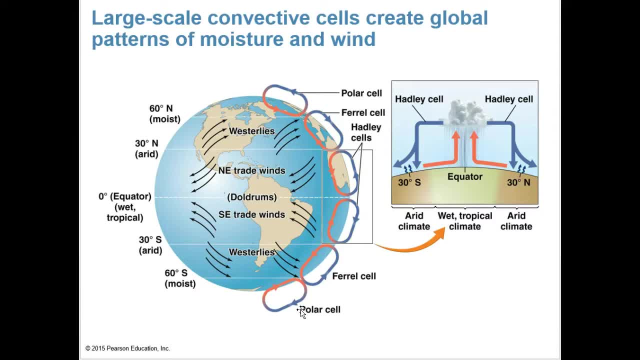 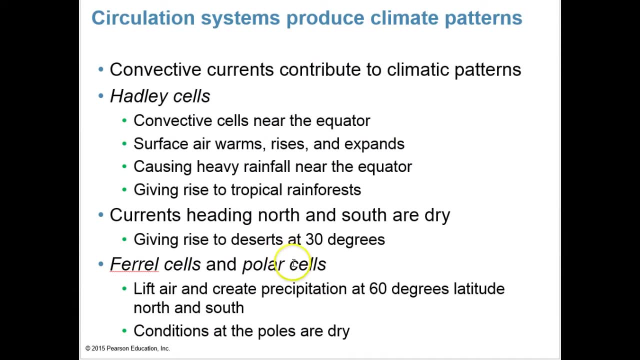 descend at 30 degrees latitude in the polar regions. Now I'll go back to our previous slide. here The pretty pairs of convective cells create wet climates near the equator, arid climates near 30 degree latitude regions and moist regions near the 60 degree latitude mark. 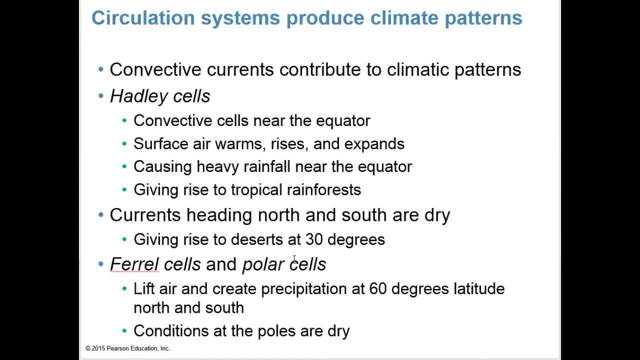 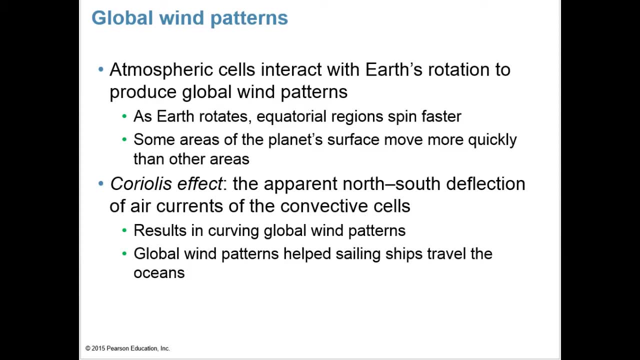 and dry regions in the poles. These patterns, with the different temperature variations, also help explain why biomes are located where they are. The Hadley, Farrell and Polar cells interact with Earth's rotation to produce our global 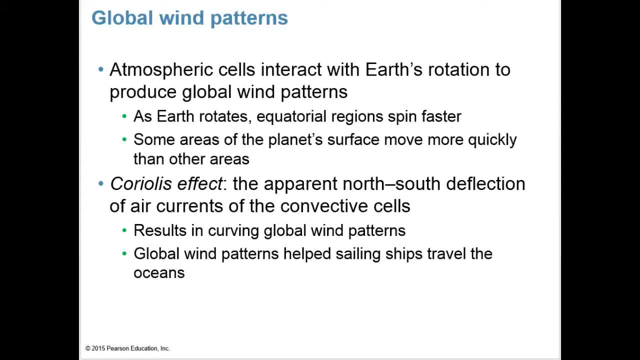 wind patterns. As the Earth rotates on its axis, regions of the planet's surface near the equator move west to east more quickly than the locations near the poles. As a result, from the perspective of an Earth-bound observer, air currents of the convective cells. 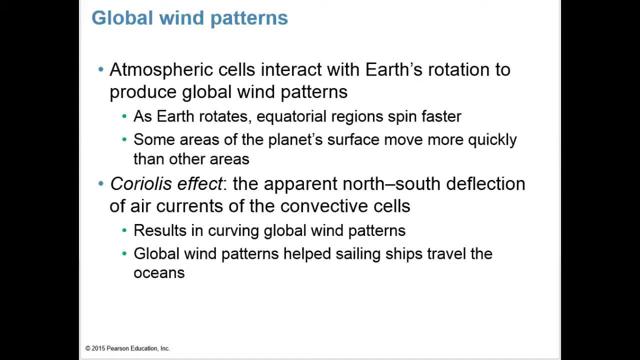 that flow north and south, appear to be deflected from a straight path. This deflection is called the Coriolis effect and results in our curving global wind patterns. It's also enabled for centuries people to use wind patterns to sail their ships. 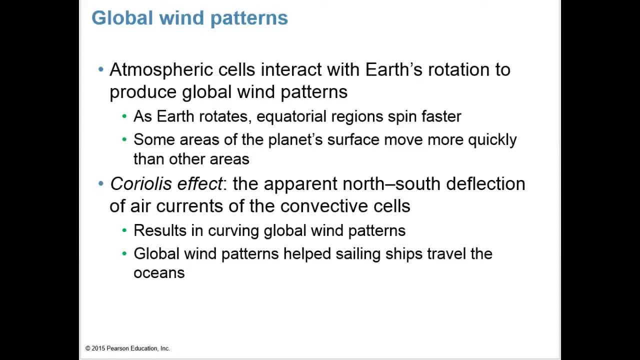 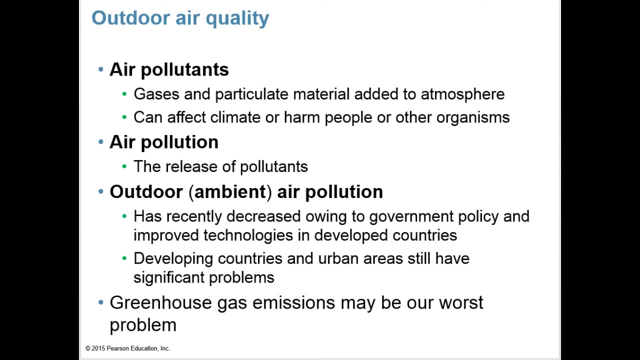 Understanding our atmosphere of course helps us understand weather and more long-range climate patterns, but it also helps us comprehend how our pollution of the atmosphere affects climate, ecological systems, economies and even human health. Throughout history, we've made the atmosphere a dumping ground for our airborne wastes. 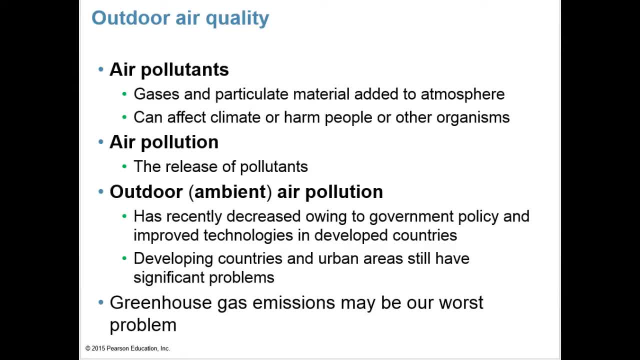 Whether from simple wood fires or modern coal-burning power plants, we've generated what's called air pollutants. These are gases and propellants. These are gases and propellants. These are particulate materials that are added to the atmosphere that can affect climate. 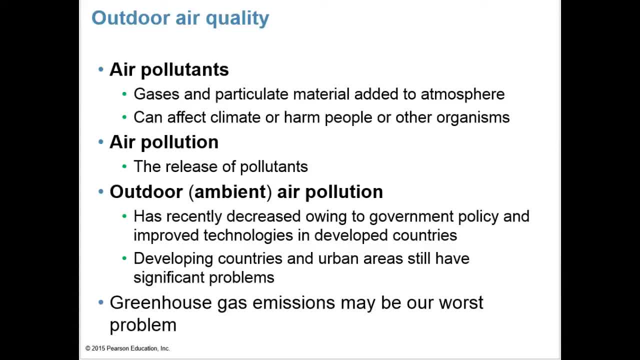 or even harm people and other organisms. Air pollution is the actual release of the pollutants. In recent decades, public policy and improved technologies have helped us reduce many types of outdoor air pollution, which is also called ambient air pollution, in industrialized nations. 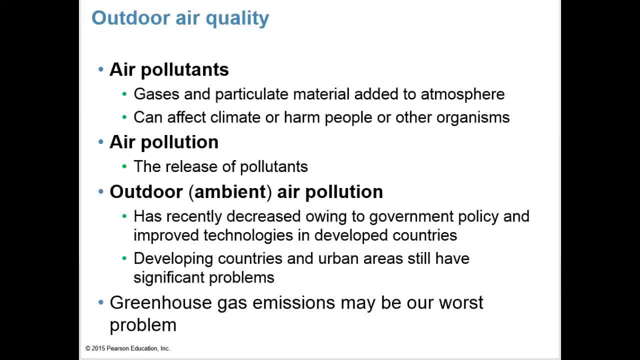 developing countries and urban areas still have significant problems. Globally, the World Health Organization estimates that 3.3 million people die prematurely each year as a result of health problems caused by outdoor air pollution. Moreover, we face an enormous air pollution challenge today in our emission of greenhouse. 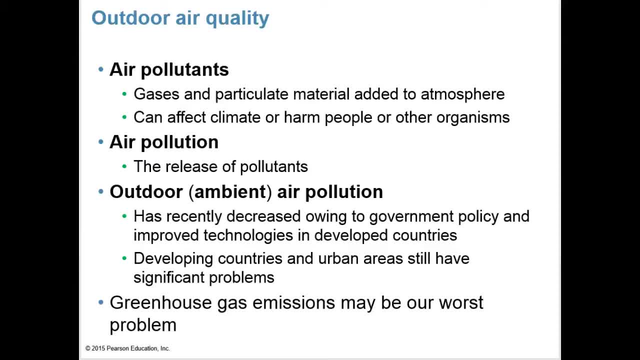 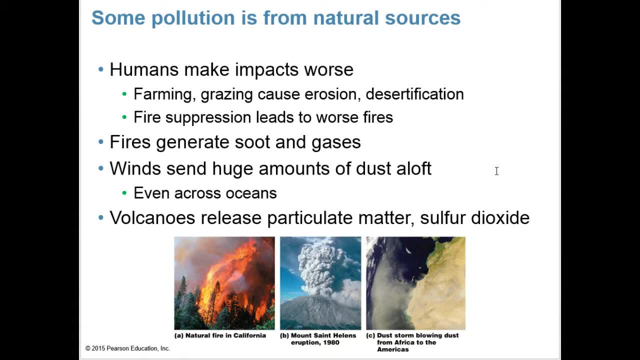 gases which contribute to global climate change. This is a real challenge. So how to deal with it? climate change and it could be our worst problem. Some pollution is actually from natural sources, but humans can make it worse by our activities, such as farming. 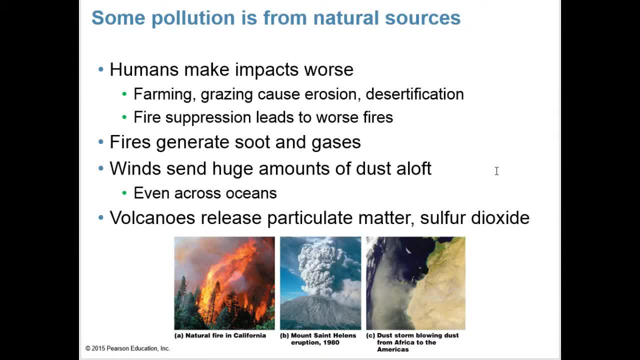 and grazing, which causes erosion and desertification. Fires can be a source of outdoor air pollution. Winds can send huge amounts of dust aloft and even across oceans, And volcanoes can even be a source of outdoor air pollution when they release their particulate matter and sulfur dioxide. Remember the point. 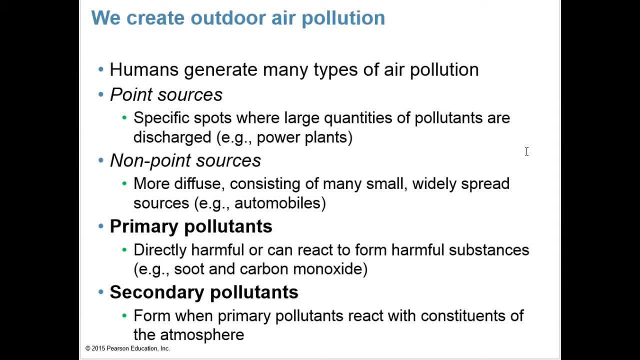 sources from our last chapter. Those are specific spots where large quantities of pollutants are discharged, such as at power plants. Non-point sources are more diffused and consistent with the air pollution that we're talking about in this video, And there are many small, widely spread sources, such as automobiles or many. 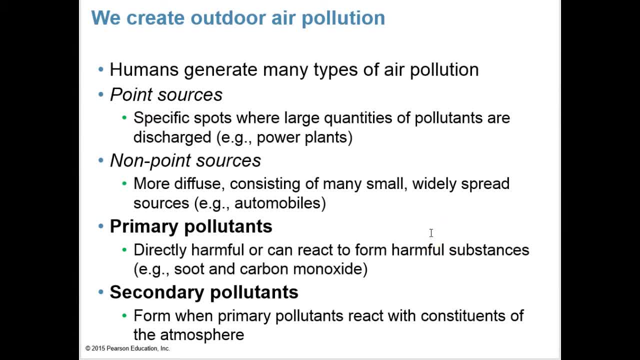 farms over a large area. Pollutants can then be broken down into two categories. Primary pollutants come directly from a source. They're directly harmful and can react to form other harmful substances. They include examples like soot and carbon dioxide. Secondary pollutants form when the primary pollutants react with constituents. 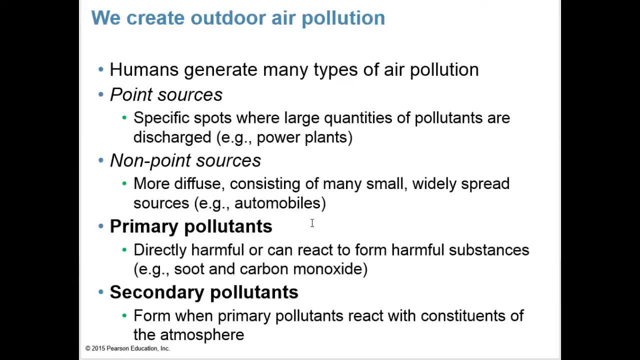 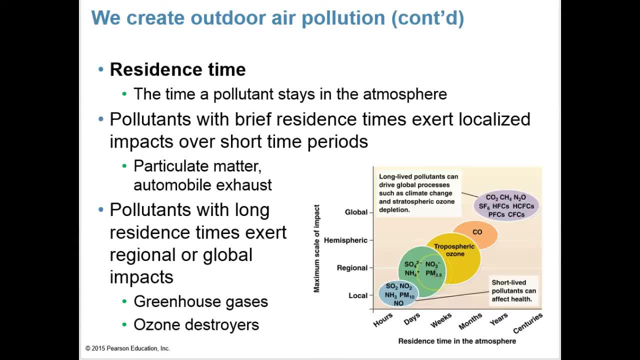 of the atmosphere. These can include things like ozone and smog. Residence time is the time a pollutant stays in the atmosphere. Pollutants with brief residence times exert localized impacts over short time periods, Such as particulate matter and automobile exhaust, But pollutants with long residence 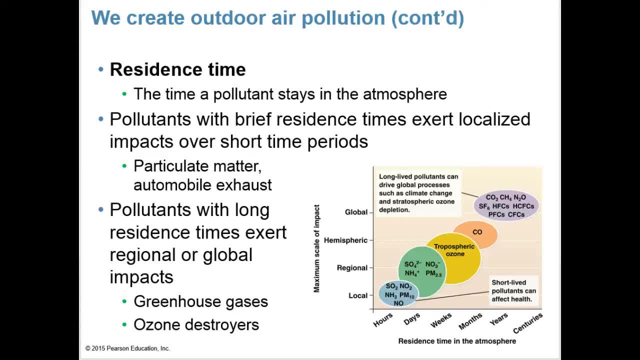 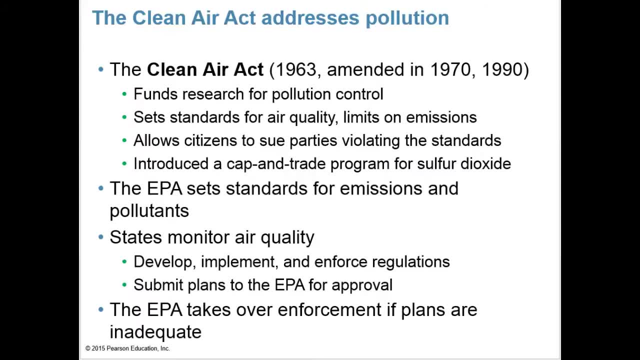 times exert regional or global impacts and include greenhouse gases and ozone destroyers. To address air pollution in the US, Congress has passed a series of laws, but most notably the Clean Air Act, which was first enacted in nineteen sixty-three but amended a few times over, particularly in nineteen, seventy and nineteen. 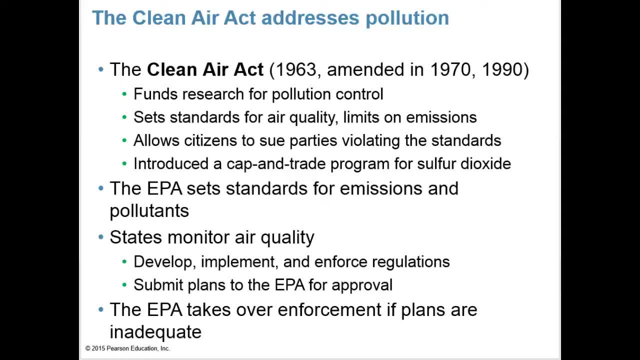 ninety. This body of legislation funds research into pollution control. It sets standards for air quality, It imposes limits on emissions from new sources and enables citizens to sue parties that violate the standards Under the Clean Air Act. the US Environmental Protection Agency, or the EPA, sets nationwide standards for emissions and for concentrations of major 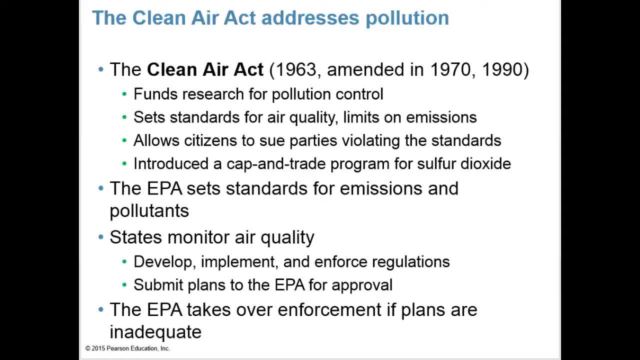 pollutants in ambient air, It's largely up to the states to monitor their emissions and air quality and to develop, implement and enforce regulations within its borders. States submit their implementation plans to the EPA, but if the state's plans are not adequate, the EPA can take control. 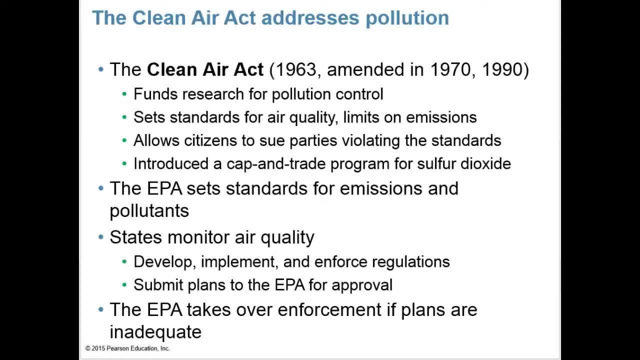 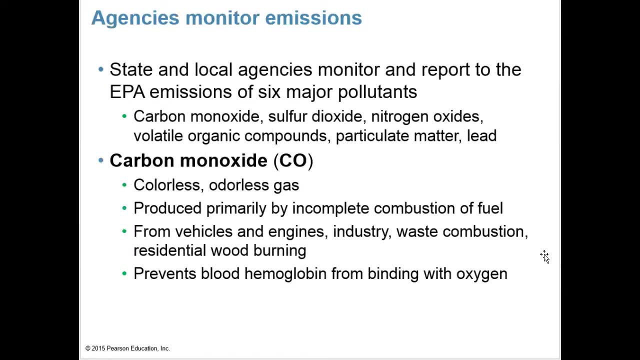 of the enforcement, And if a region fails to clean up its air, the EPA can prevent it from receiving federal money for transportation projects. as punishment, State and local agencies monitor and report to the EPA emissions of six major pollutants: Carbon monoxide, sulfur dioxide. 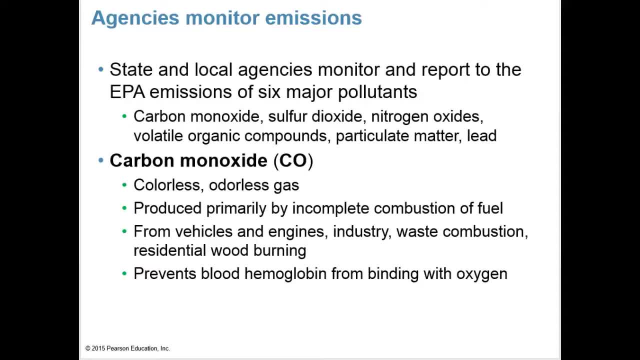 nitrogen oxides, volatile organic compounds, particulate matter and lead. Carbon monoxide is a colorless, odorless gas. It's produced primarily by incomplete combustion of fuel. It's from vehicles and engines, industry waste combustion and residential wood burning In too much amounts for living organisms. it can prevent blood hemoglobin from binding with oxygen. 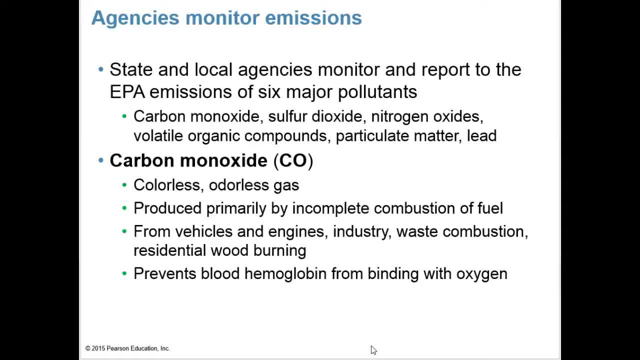 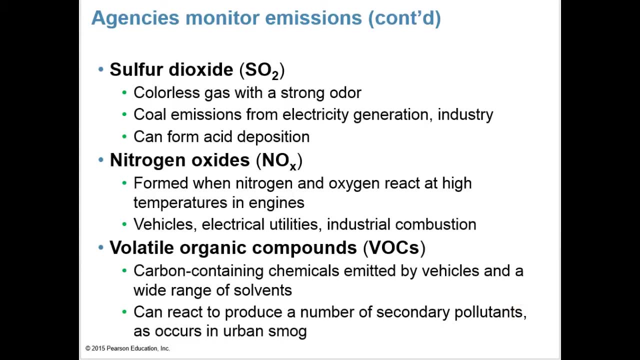 And therefore it can be very deadly. It induces nausea, headaches, fatigue, heart and nervous system damage and then potentially death. Sulfur dioxide is a colorless gas with a strong odor. If you've smelt rotten eggs, you've smelt sulfur dioxide. It comes from coal, emissions, from electricity generation and from industry And can be used to produce carbon dioxide. 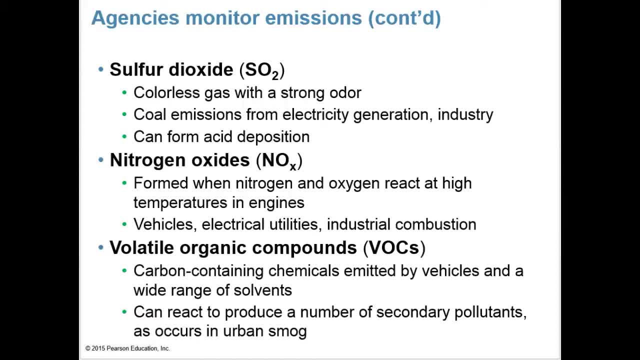 It can contribute to forming acid deposition Nitrogen oxide, often nicknamed NOX because it can come in the form of NO2 or NO3,. it's formed when nitrogen and oxygen react at high temperatures in engines From vehicles, electrical utilities. 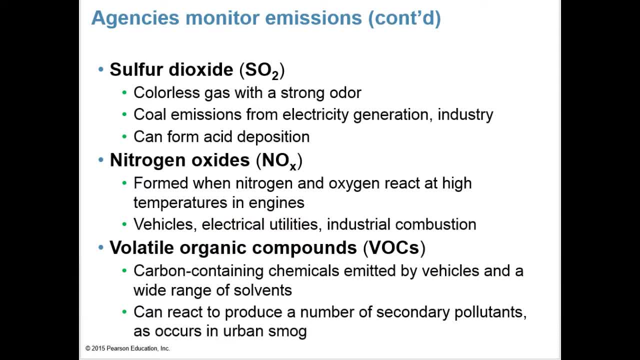 and industrial combustion Public//. kaikki Nitrogen emissions contribute to smog, acid deposition and stratospheric ozone depletion. Volatile organic compounds, also called VOCs for short, are carbon containing chemicals emitted by vehicles and a wide range of solvents. 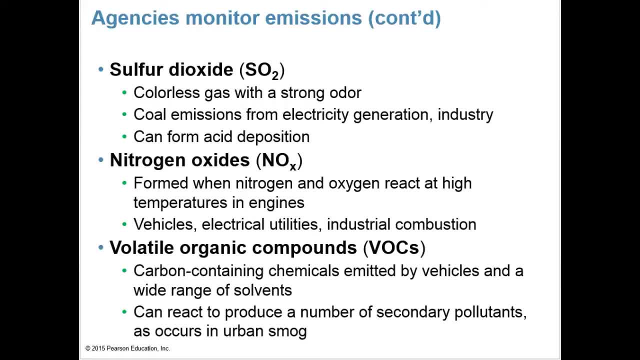 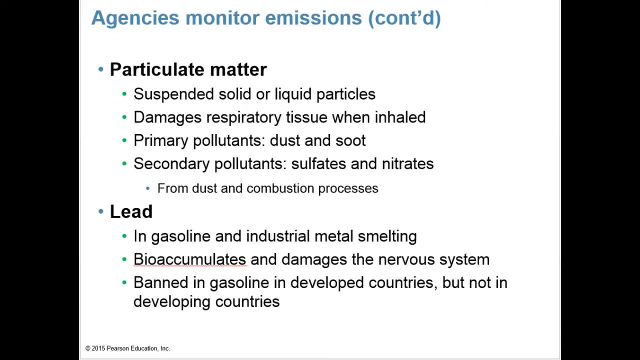 And they can react to produce a number of secondary pollutants and occur as urban smog. Particulate matter is suspended solids or liquid particles in the atmosphere. It can damage respiratory tissue when inhaled, And the ones that are called primary pollutants are dust and soil. 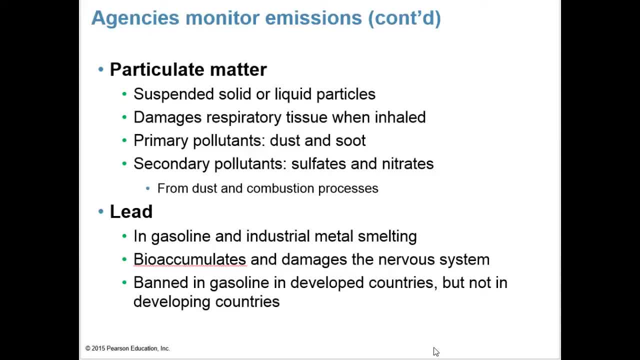 Soot and secondary pollutants, remember, react when primary pollutants combine with other things in the atmosphere. Those include sulfates and nitrates from the dust and combustion processes. Lead is a heavy metal that enters the atmosphere as a particulate pollutant. You can find it in gasoline and industrial fuel. 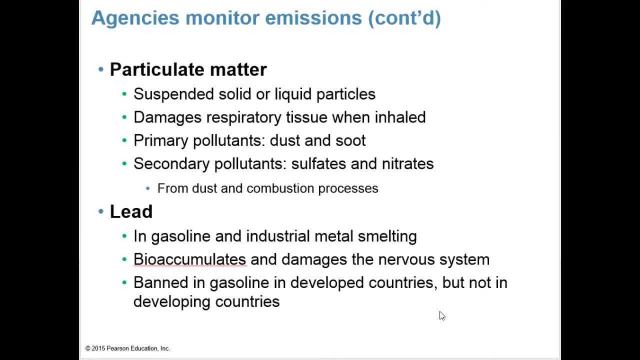 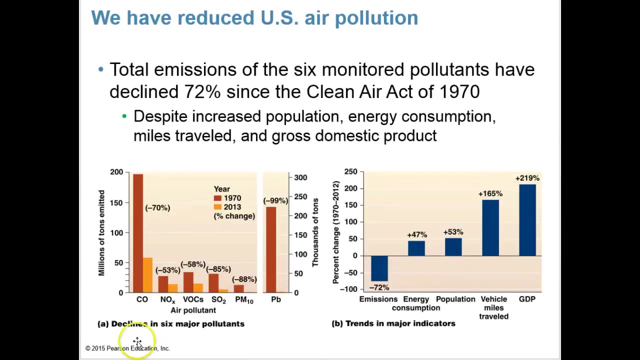 Also metal smelting. It bioaccumulates, remember. that's when it builds up in your body And it then can lead to damage of the nervous system. It's banned now in gasoline in developed countries like the United States, But not in developed countries. 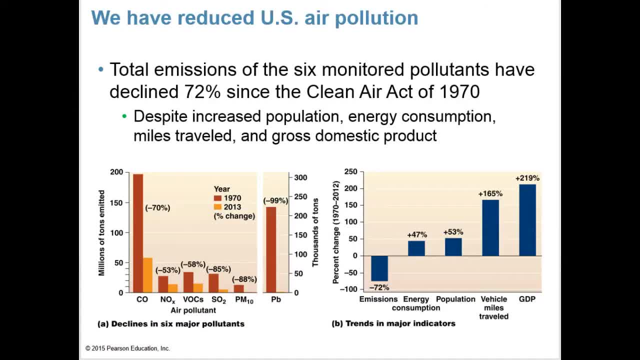 Since the Clean Air Act of 1970, the US has reduced emissions of each of the six monitored pollutants substantially, In fact by 72%. These dramatic reductions in emissions have occurred despite significant increases in the nation's population energy consumption. 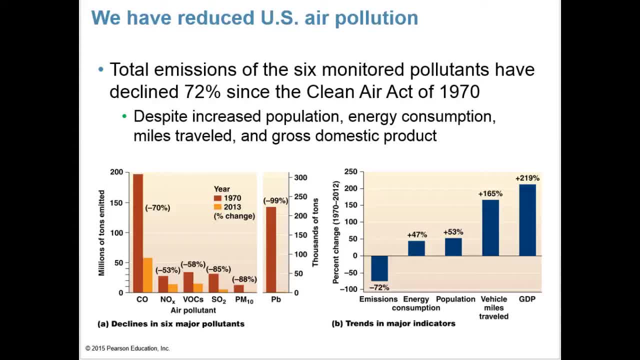 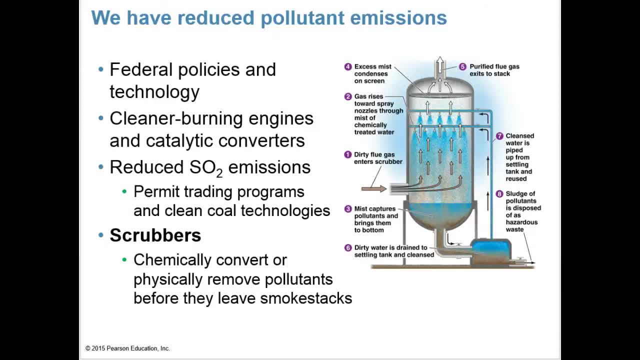 and miles traveled by vehicles and gross domestic product. These the success with the Pollution Control Act. the pollution control is thought to be one of the top accomplishments of the United States in safeguarding human health and environmental quality. The EPA estimates that between 1970 and 1990,. 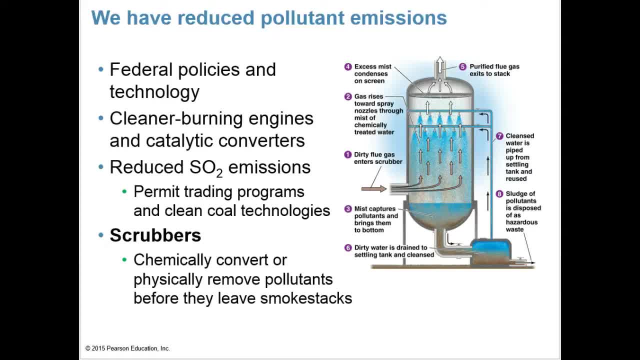 cleaner air saved the lives of 200,000 Americans. The success in controlling pollution has come as a result of policy steps and technological developments In factories, power plants and refineries- technologies like baghouse filters, electrostatic precipitators and scrubbers. 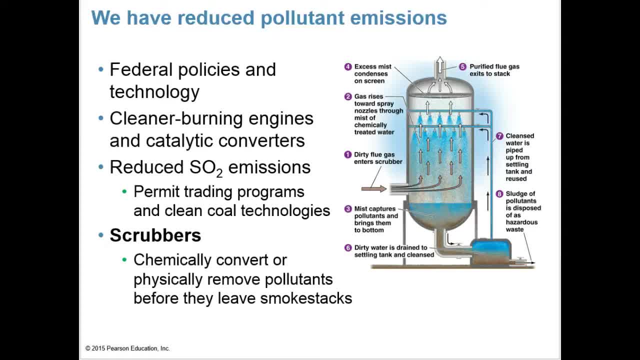 chemically convert or physically remove pollutants before they're actually emitted from smokestacks. Here over to the right, we can see a scrubber at work. Typically, a scrubber can remove at least 90% of the particulate matter and gases like sulfur dioxide. 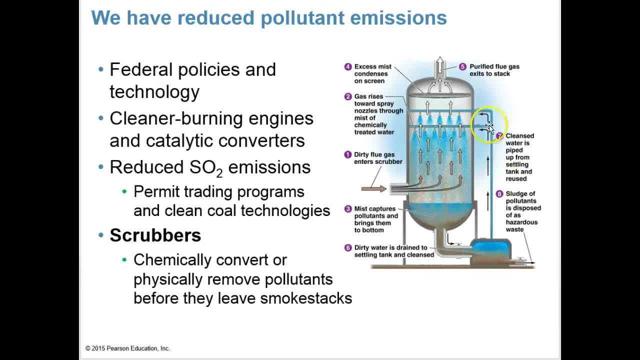 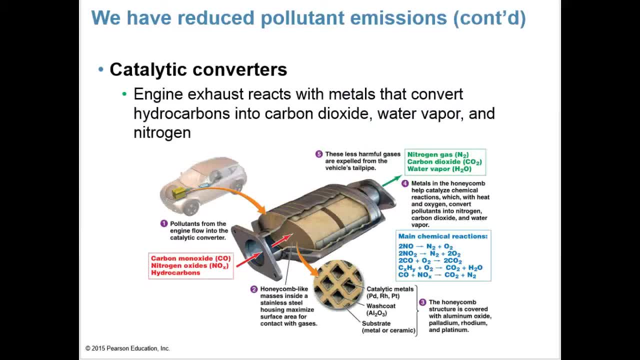 They come in many designs. This one's called the Spray Tower Scrubber. Cleaner-burning motor vehicle engines and automotive technologies like the catalytic converter have also played a large part in helping us to clean up our air. A catalytic converter as shown here in the diagram. 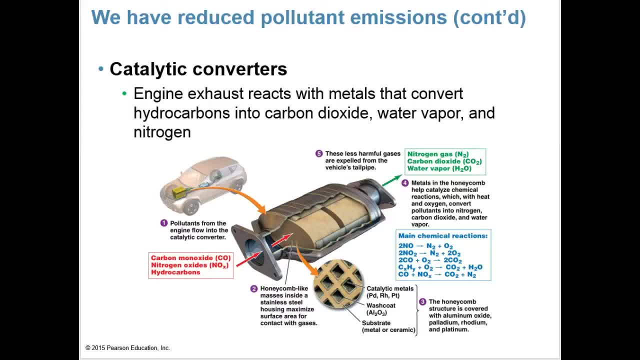 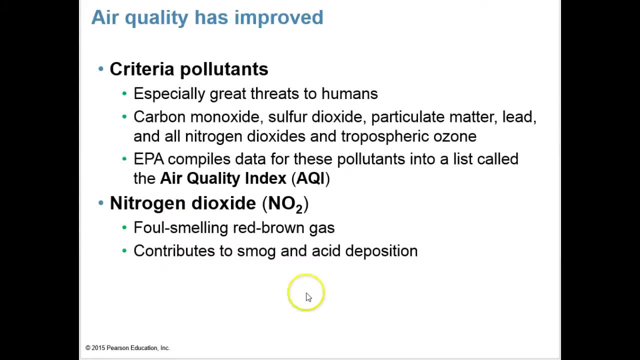 the engine exhaust reacts with metals that convert hydrocarbons, and also including carbon monoxide and other nitrogen compounds. It converts them into carbon dioxide, water vapor and nitrogen gas. As a result of emissions reductions, air quality has improved markedly in industrialized nations. 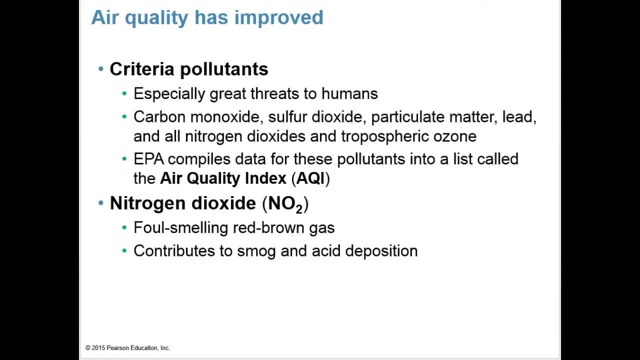 like the US, The EPA here and the states monitor outdoor air quality by measuring concentrations of six criteria pollutants, and those are ones that are established to be a threat to human health. The six criteria pollutants include four of the six pollutants whose emissions are monitored. 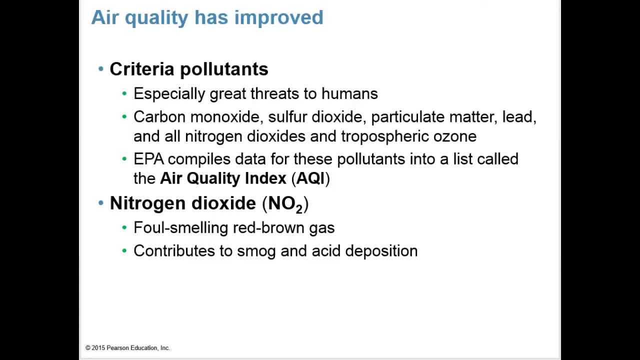 Carbon monoxide, sulfur dioxide, particulate matter and lead, and all nitrogen dioxide and tropospheric ozone. Across the US, over 4,000 monitoring stations take hourly or daily samples of air and then share their data on pollutant concentrations with the EPA. 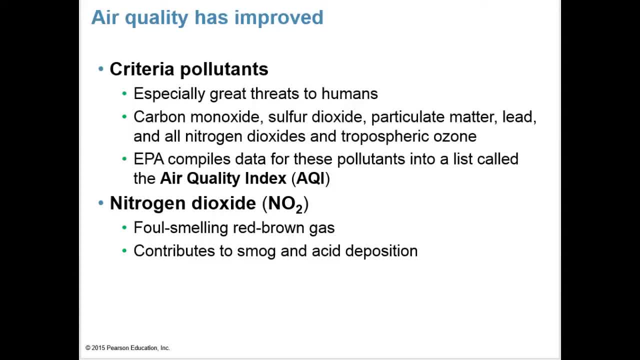 The EPA then compiles the data and calculates what's called the Air Quality Index or the AQI. For each site And each of the six criteria pollutants receives an AQI on a value of 0 to 500 that reflects its current concentration. 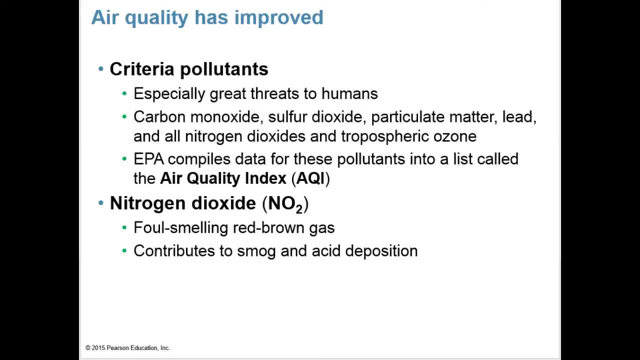 If a value is below 100, it's deemed satisfactory, but above 100 is indicating unhealthy conditions. People in Los Angeles, for instance, breathe air that violates health standards for five of the six criteria pollutants. One of the criteria pollutants is nitrogen dioxide- NO2.. 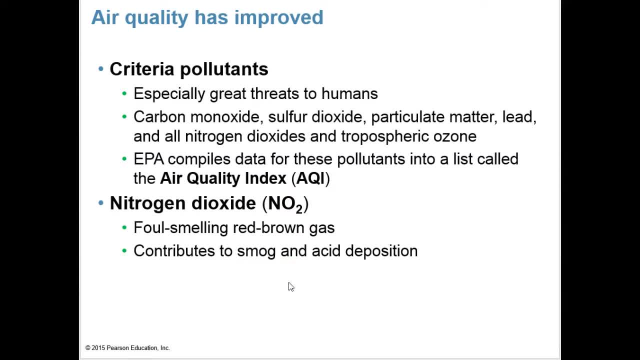 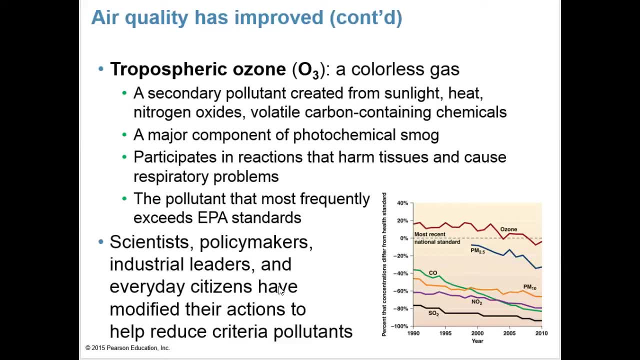 It's a foul-smelling red-brown gas and is one that contributes to smog and acid deposition. Tropospheric ozone is a colorless gas, also known as O3. It's a secondary pollutant created from the interaction of sunlight. 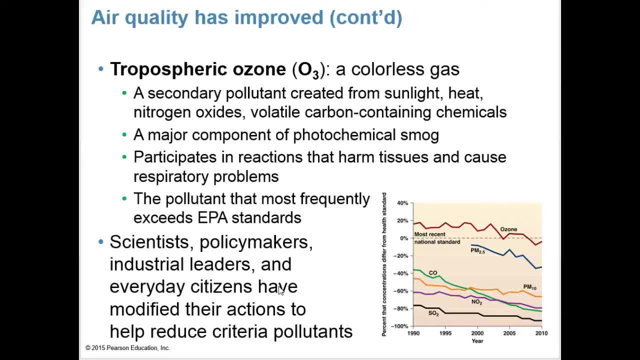 heat, nitrogen oxides and volatile carbon-containing chemicals- Remember VOCs, A major component of photochemical smog. It participates in reactions that harm tissues and cause respiratory problems, And it's the pollutant that most frequently exceeds EPA standards. Scientists, policymakers, industrial leaders and everyday citizens. 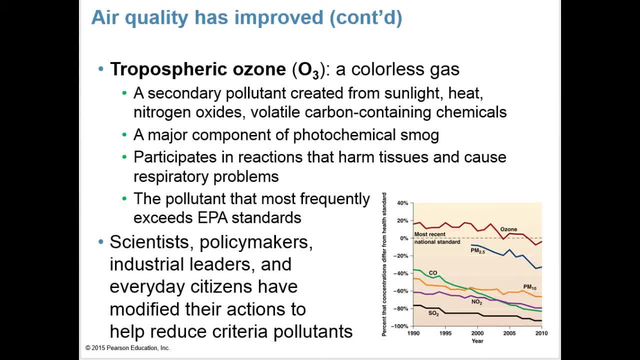 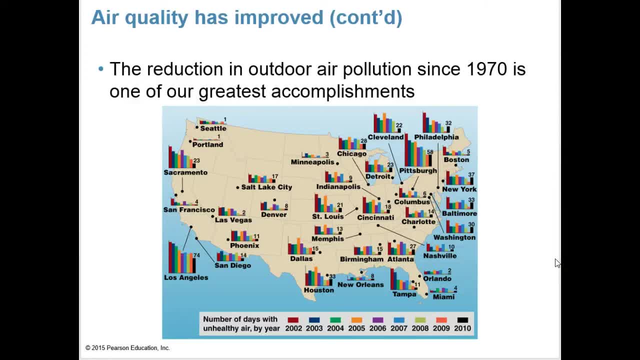 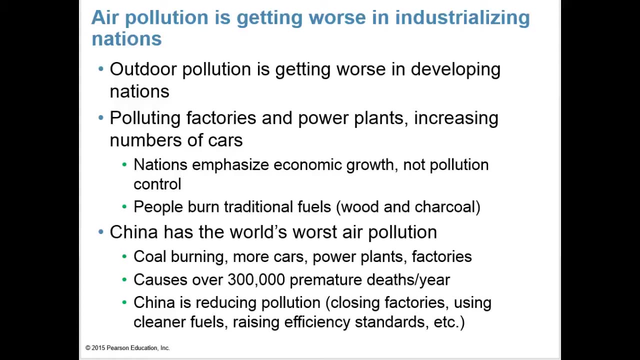 have modified their actions to help reduce criteria pollutants, And the reduction in outdoor air pollution since 1970 is one of our greatest accomplishments. in the US, Outdoor air pollution is getting worse in developing countries, Polluting factories and power plants and increasing numbers of cars. 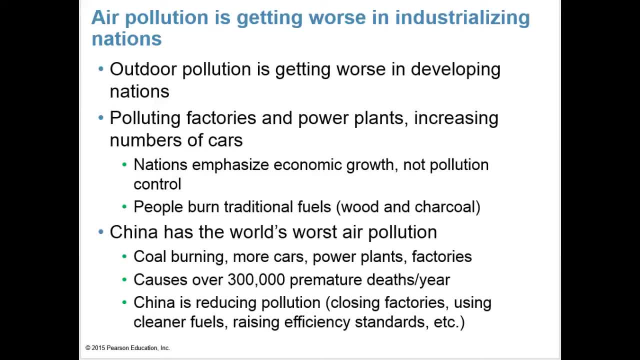 all contribute to our air pollution problem. Nations emphasize economic growth, not pollution control, when they're developing, And people burn traditional fuels like wood and charcoal, which also contributes to the air pollution problem, which also contributes to the air pollution problem. China has the world's worst air pollution. 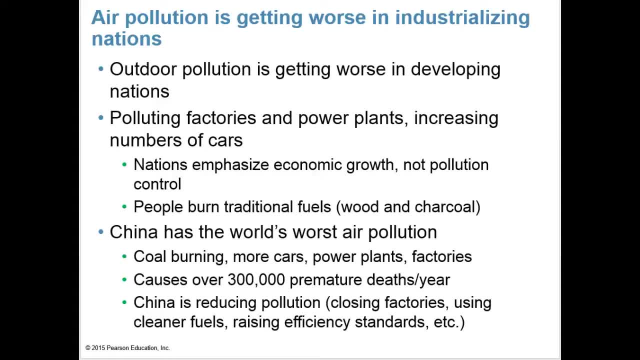 It has more coal burning, more cars, power plants and factories and causes over 300,000 premature deaths per year. China is reducing its pollution by closing factories and using cleaner fuels and higher standards, but still has a long way to go. 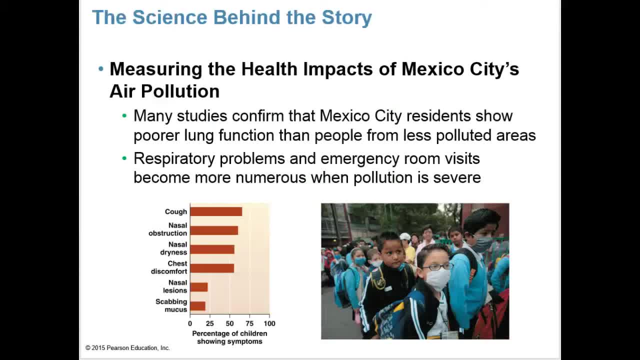 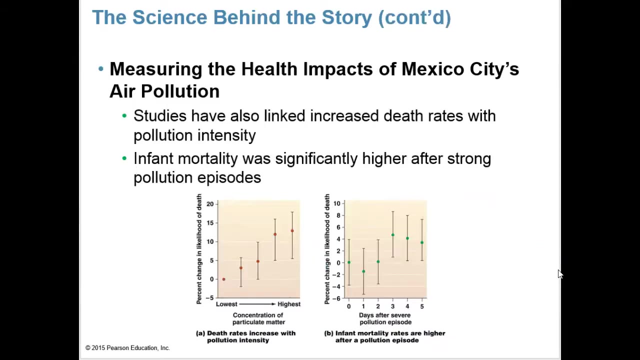 Studies have been done to measure the impacts of air pollution on human health, especially in Mexico City, And respiratory problems and emergency room visits are one of the factors that can be used to measure this. They've become more numerous when pollution is severe. Studies have also linked increased death rates with pollution intensity. 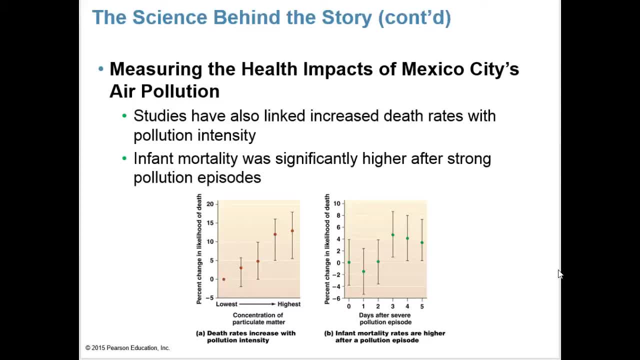 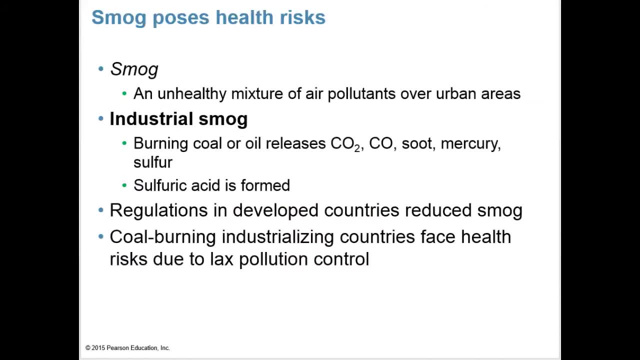 Unfortunately, infant mortality was significantly higher after the stronger pollution episode than Mexico City. Smog is an unhealthy mixture of air pollutants over urban areas. Industrial smog comes from burning coal or oil and it releases carbon dioxide and carbon monoxide, soot and even mercury and sulfur. 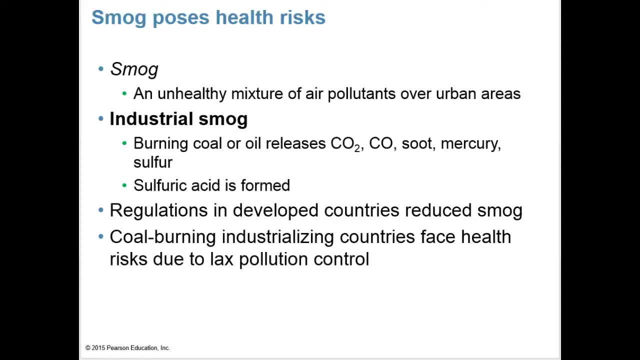 And this can contribute to the formation of sulfuric acid Regulations in developed countries- has reduced smog, but, as we've said before, developing countries have more problems yet, and coal burning industrializing countries face health risks due to their lax pollution control measures. 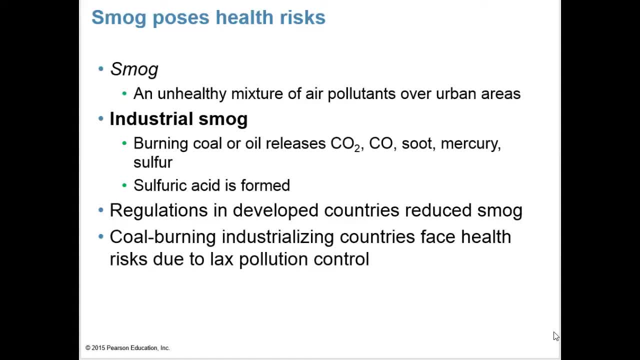 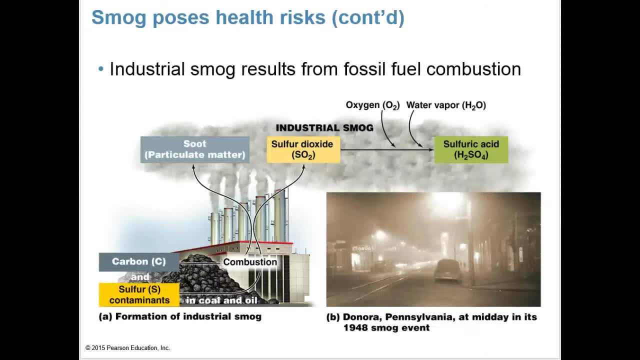 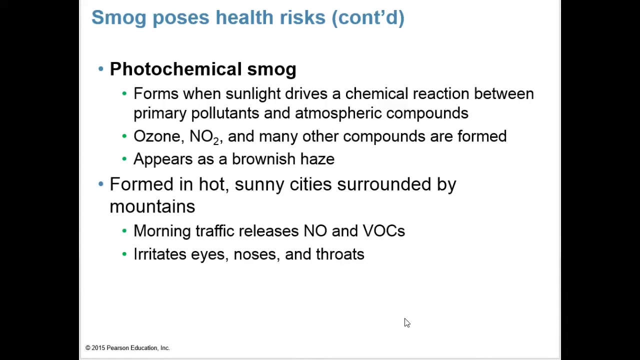 They're thinking to bring up the economy, not to increase or not to decrease pollutants, but to reduce them. Here we can see a picture in Denora, Pennsylvania, at midday in a 1948 smog event. Photochemical smog forms when sunlight drives a chemical reaction. 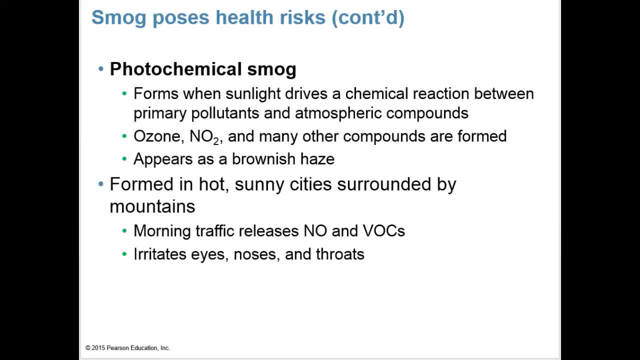 between primary pollutants and atmospheric compounds. It forms ozone and nitrogen compound and other compounds and can appear as a brownish haze. This is typically formed in hot, sunny cities surrounded by mountains and especially in morning traffic that releases nitrogen oxide and VOCs. 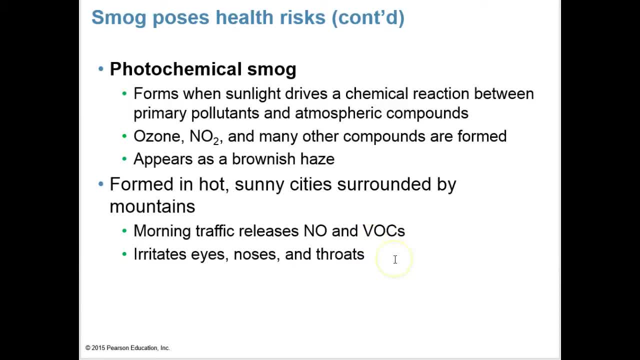 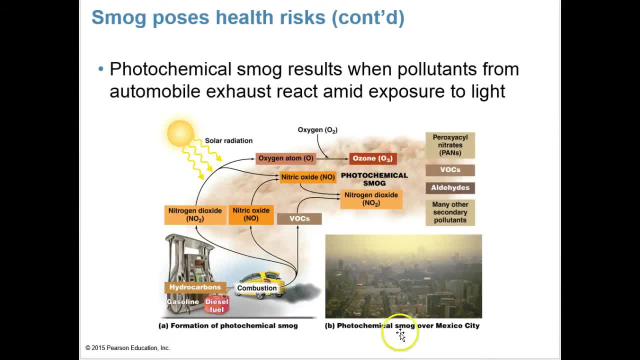 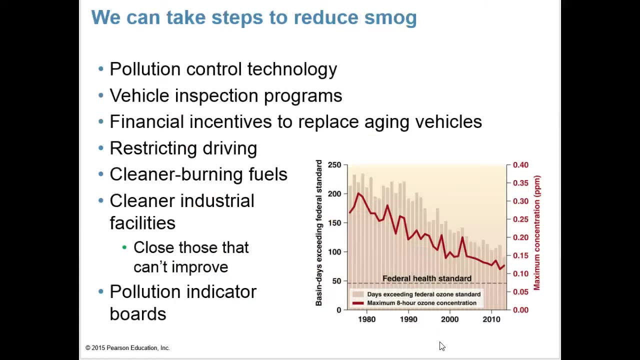 This can be an irritant for eyes and noses and throats of humans. Here we can see a picture of photochemical smog: Photochemical smog over Mexico City. We can take steps to reduce smog, such as pollution control technology. 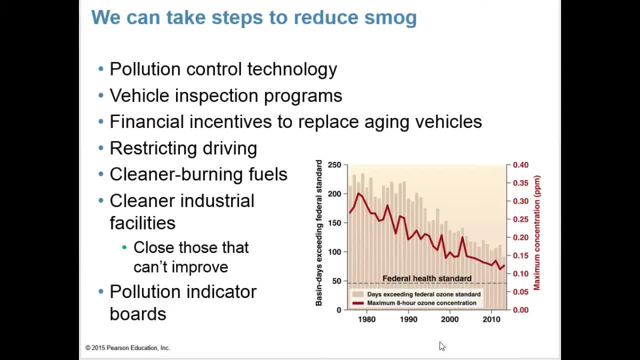 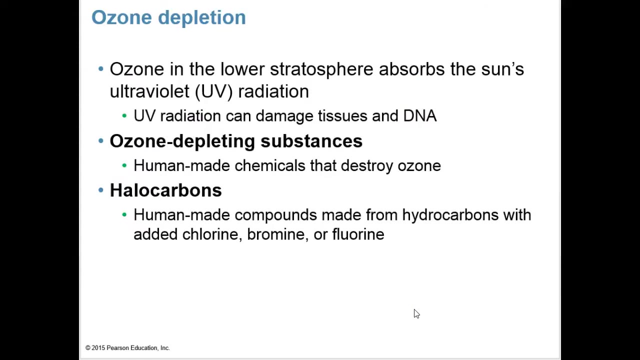 vehicle inspection programs, financial incentives to replace aging vehicles, restricting driving, cleaner burning fuels, cleaner industrial facilities and close those that won't improve and buy pollution indicator boards. Although ozone in the troposphere is a pollutant in photochemical smog. 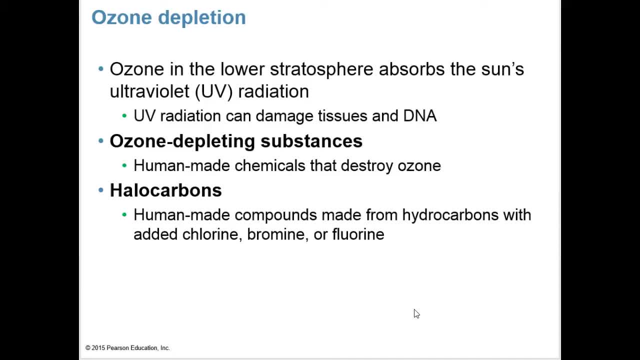 ozone in the stratosphere protects life on Earth by absorbing sun's UV light, which, as we've already said, can damage human tissue and DNA. When scientists discovered that our planet's stratospheric ozone was being depleted, they realized this posed a major threat. 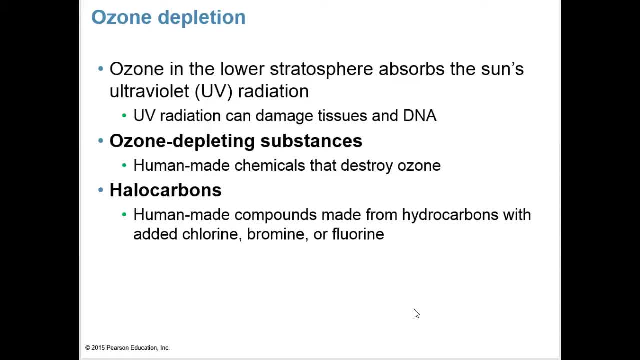 to human health and the environment, and years of research by hundreds of scientists revealed that certain airborne chemicals destroy ozone and that most of these ozone-depleting substances are actually human-made. Halocarbons are one of these. These are human-made compounds. 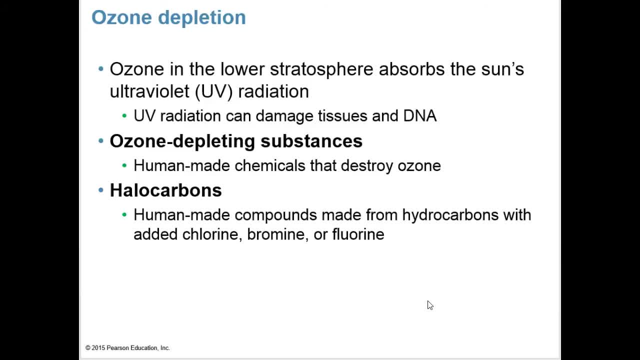 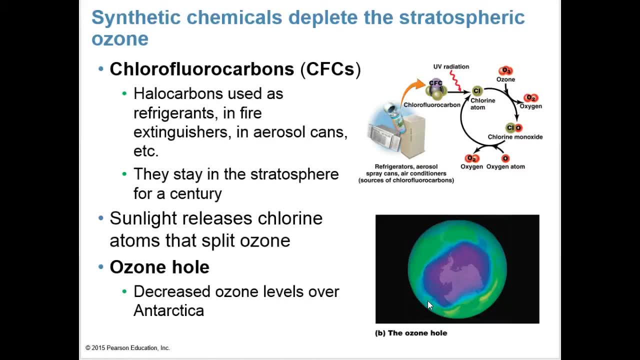 from hydrocarbons with added chlorine, bromine and fluorine. Chlorophorocarbons, or CFCs are halocarbons used as refrigerants in fire extinguishers and in aerosol cans and can stay in the stratosphere for centuries. 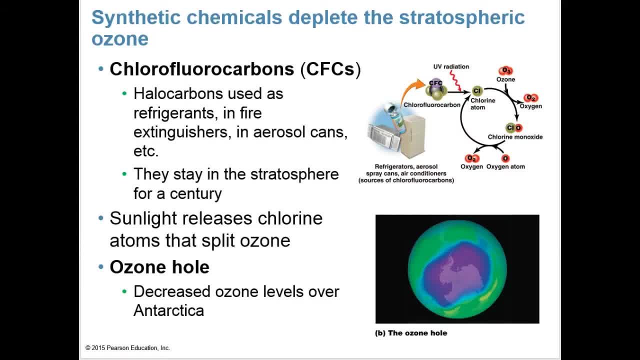 They work like this. in the atmosphere where there's intense UV radiation from the sun, There's a two-step chemical reaction that occurs: UV radiation breaks the bonds in the CFC molecules, which release their chlorine atoms, and then each newly freed chlorine atom can split an ozone molecule. 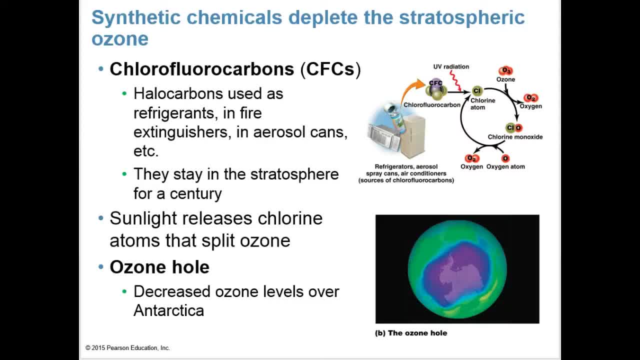 and then ready itself to split more. During its long residence time, each free chlorine atom can catalyze the destruction of as many as 100,000 ozone molecules. The ozone hole is the decreased ozone level over the Antarctica area. This was announced in 1985,. 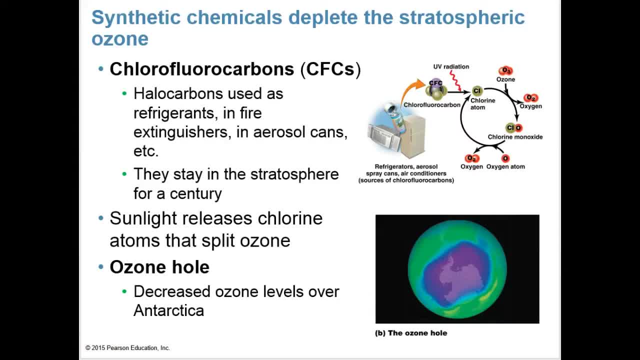 and researchers shocked the world by announcing that the stratospheric ozone levels over Antarctica in the southern springtime had declined by nearly half than during the previous decade. That leaves a thinned ozone concentration that was soon nicknamed the ozone hole. It took a lot of detective work to find out. 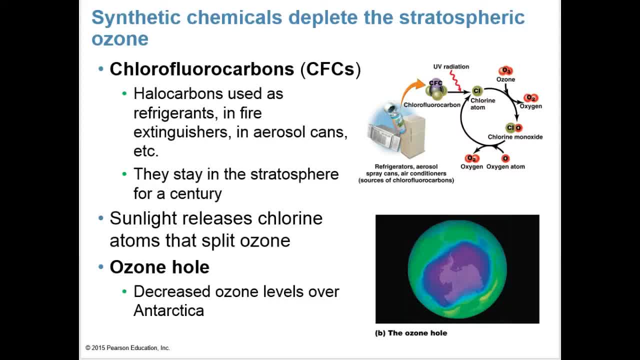 why that actually happens most severely over Antarctica. It happens elsewhere as well, but seems to be most severe and seasonal over Antarctica. During the dark and frigid Antarctic winter, clouds form in the stratosphere containing condensed nitric acid, which can split chlorine atoms off from CFCs. 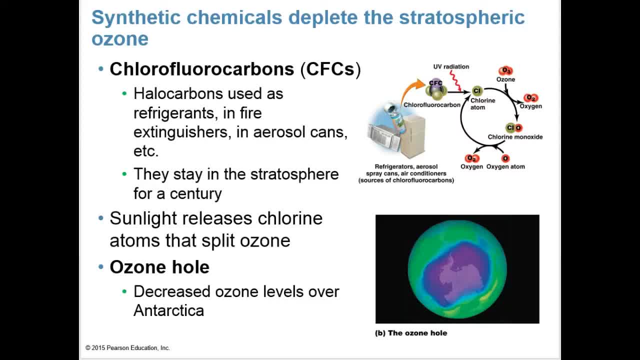 The freed chlorine atoms then accumulate in the clouds trapped over the Antarctic by circular wind currents. In the Antarctic spring, which starts in September, sunshine returns and dissipates the clouds, which releases the chlorine atoms which then begin destroying ozone. The solar radiation there also catalyzes the chemical reactions. 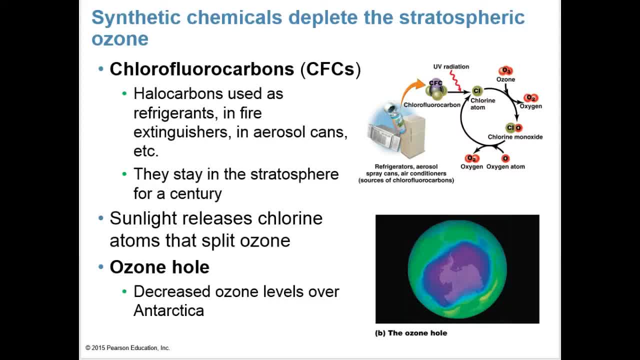 and speeds up the depletion as the temperatures warm. The hole lingers over Antarctica until December, When warm it weakens the circular currents, allowing ozone-depleted air to diffuse away and ozone-rich air from elsewhere to stream in. The ozone hole vanishes then again until the following spring. 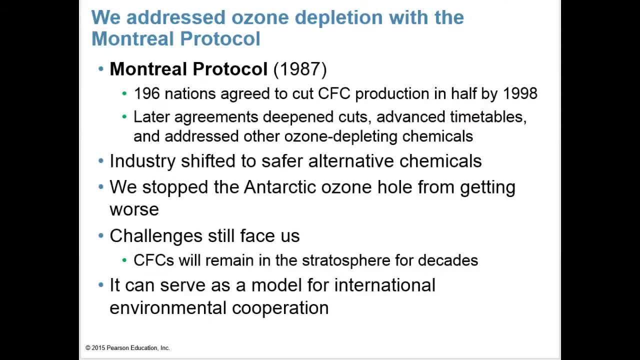 We've addressed the ozone depletion with what's called the Montreal Protocol in 1987. 196 nations agreed to cut CFC production in half by 1998.. Later agreements deepened the cuts, advanced the timetables and addressed other ozone-depleting chemicals. 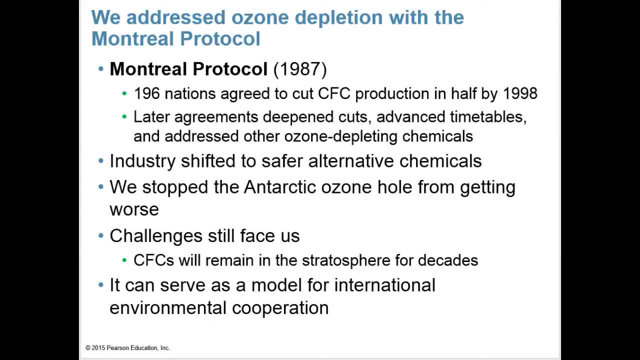 Industries have shifted to safer alternative chemicals And we've stopped the Antarctic ozone hole from getting worse. But the challenges still face us because CFCs can remain in the stratosphere for decades And, as we know, those chlorines can go on to damage more and more ozone. 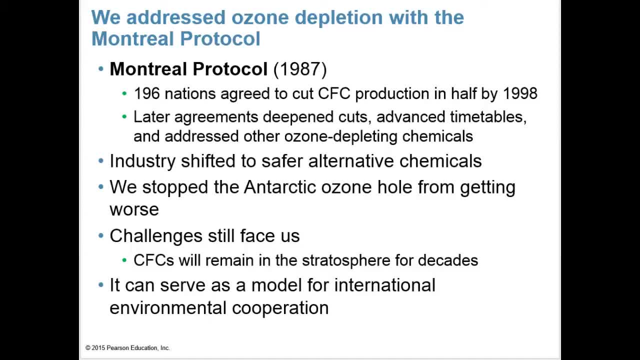 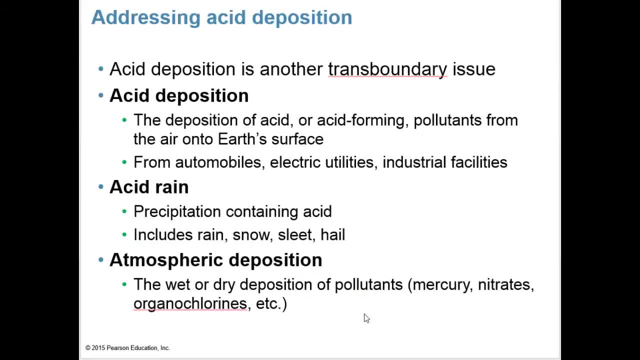 It can serve as a model for international environmental cooperation, though, and that's good news. Acid deposition is another transboundary issue, just like ozone was, And what this means is that it's not just a problem of one country, because this is occurring from our atmosphere. 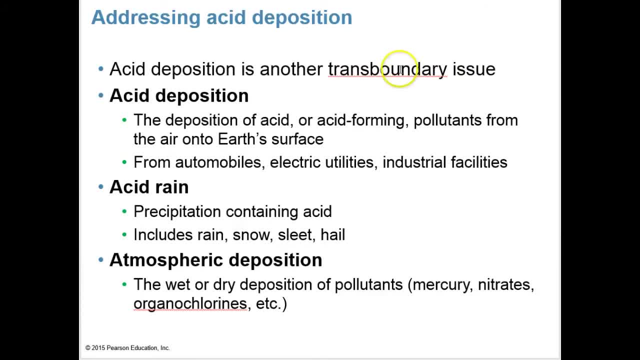 It's a global issue, So many countries need to take issue and take note with this and work together. Acid deposition is the deposition of acid or acid-forming pollutants from the air onto Earth's surface. It can come from automobiles, electric utilities. 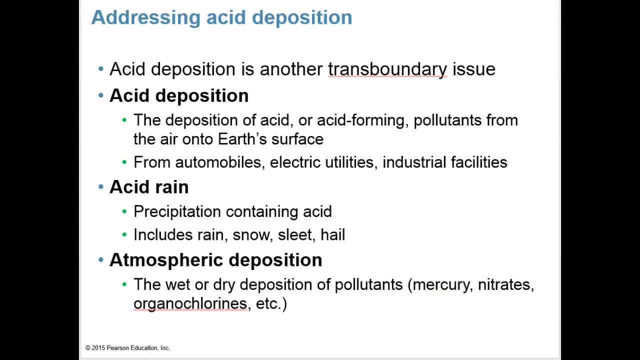 and industrial facilities. Often acid deposition can fall as acid rain, which is precipitation containing acid. It can include not just rain, but also snow, sleet and hail. Acid deposition is one type of atmospheric deposition which refers broadly to the wet or dry deposition. 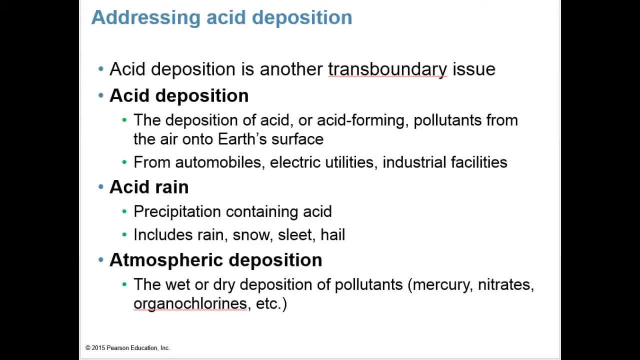 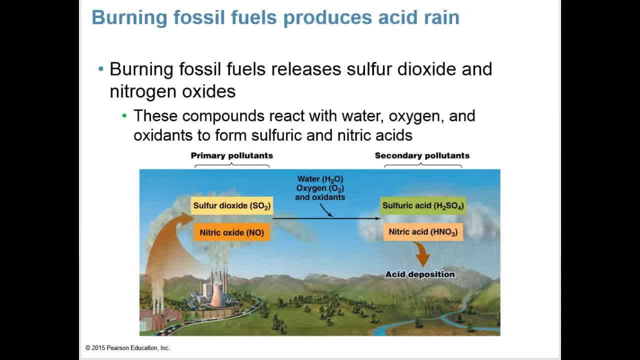 of a variety of pollutants, including mercury, nitrates, organochlorines and other pollutants. Burning fossil fuels releases sulfur dioxide and nitrogen oxides into the atmosphere, and these compounds in the atmosphere then can react with water and oxygen and other oxidants to form sulfuric and nitric acids. 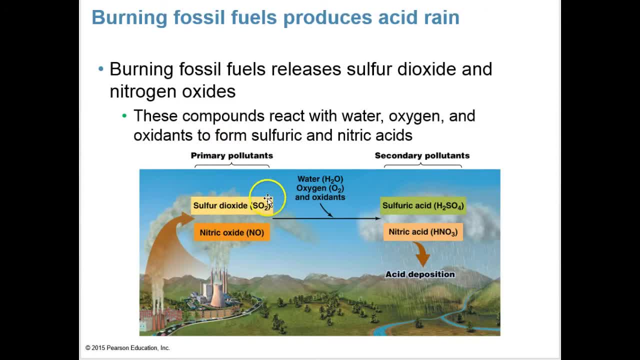 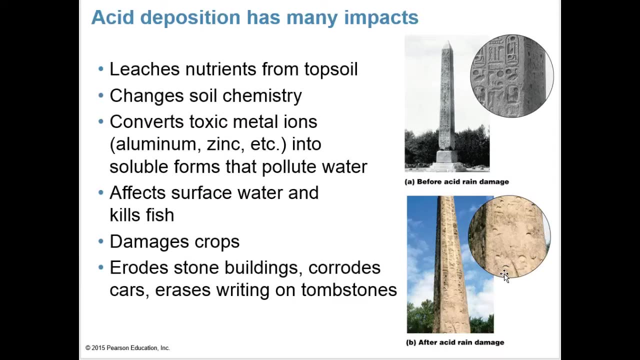 So here we have our primary pollutants and after their reaction with constituents of the atmosphere, we get our secondary pollutants. Acid deposition has many impacts. It can leach out nutrients from topsoil and change our soil chemistry. It can convert toxic metal ions like aluminum and zinc into soluble forms. 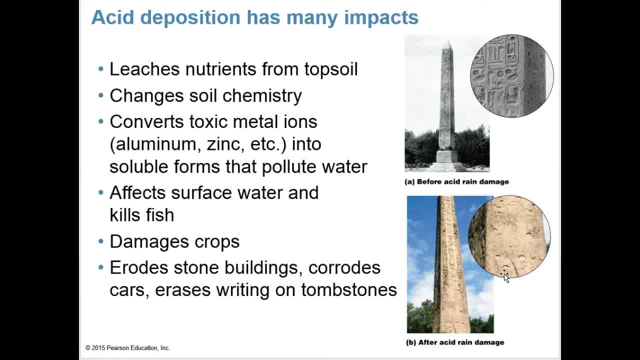 that can go on to pollute our water, which then would affect surface water and kill fish. It can damage our crops and even erode stone buildings and corrode cars and even erase writing on tombstones, like we see in the diagram here. 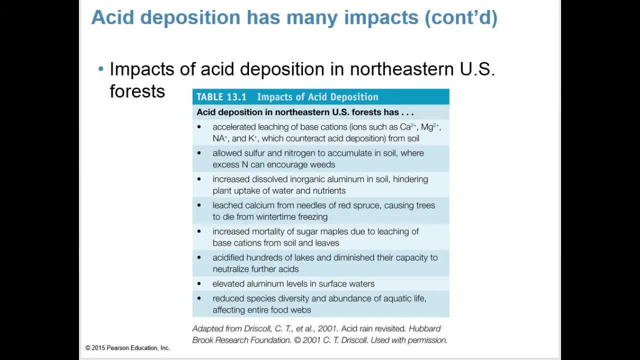 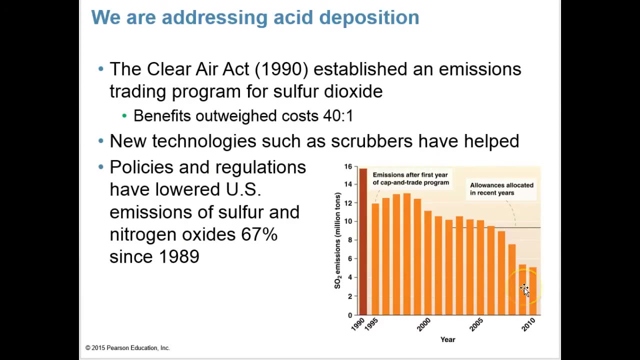 Here's a list of some acid deposition in northeastern US forests, of how that's happening. We're addressing acid deposition. The Clean Air Act of 1990 established an emissions trading program for sulfur dioxide and the benefits outweighed the costs- 40 to 1.. 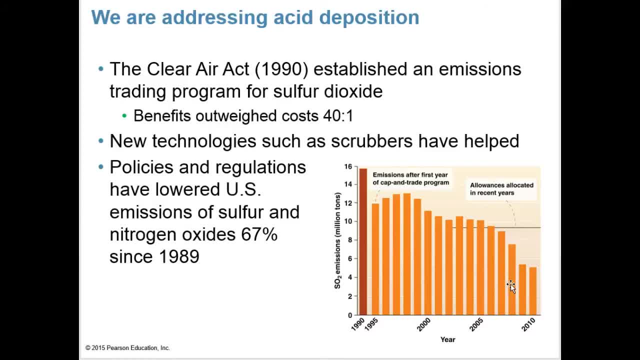 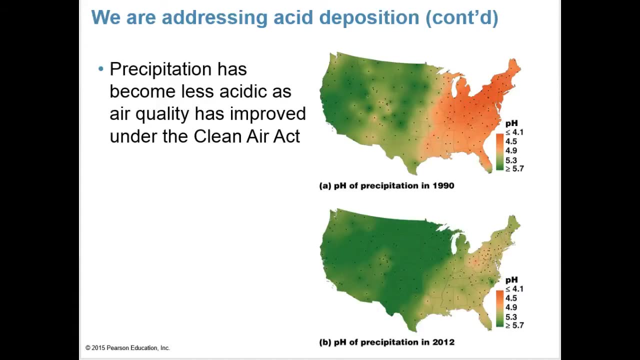 New technologies like the scrubbers we've talked about in industry have helped. Policies and regulations have lowered US emissions of sulfur and nitrogen oxides by 67% since 1989. Precipitation has become less acidic as air quality has improved. 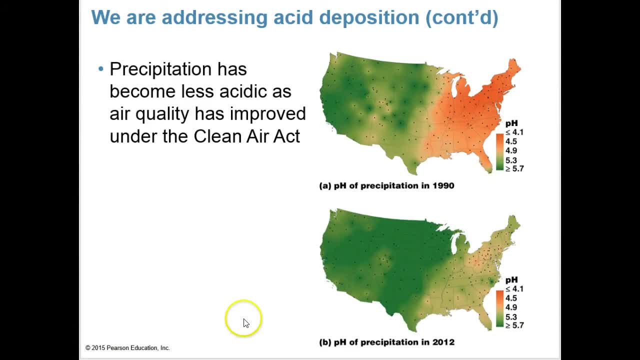 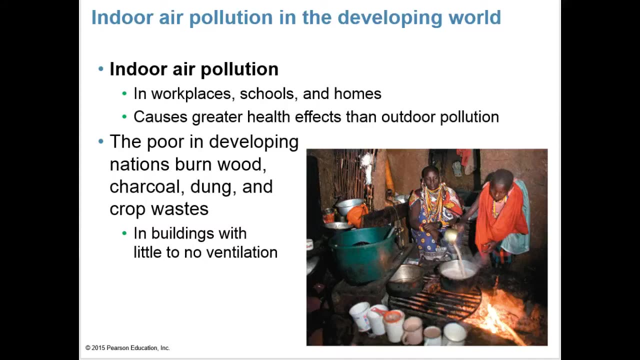 under the Clean Air Act, as we can see here in these charts From 1990 to 2012,. a big improvement has been made. Though much of this chapter has been about outdoor air pollution, indoor air pollution can be a big problem as well. 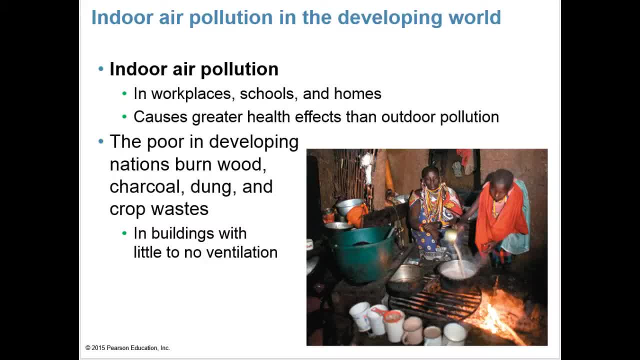 Indoor air generally contains higher concentration of pollutants than does the outdoor air and, as a result, the health impacts from indoor air pollution in workplaces, schools and homes outweigh those from outdoor air pollution. The World Health Organization attributes nearly 3.5 million premature deaths. 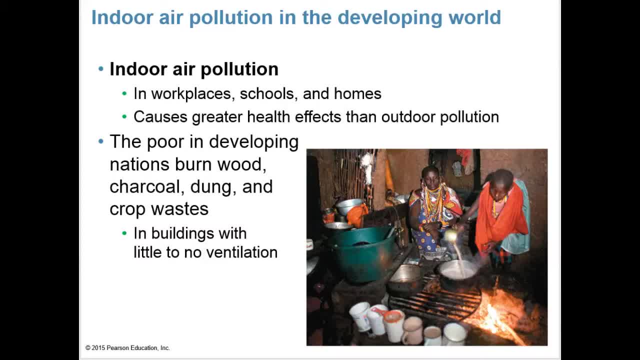 each year to indoor air pollution, compared with 3.3 million for outdoor. It's thought that indoor air pollution takes nearly 10,000 lives each day. If it seems surprising, consider that the average US citizen spends at least 90% of their time indoors. 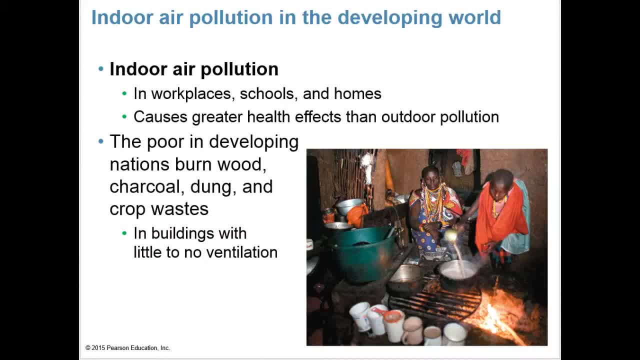 And the things that surround you can have different pollutants and synthetic substances, such as cleaning products that you use in your home or office, the carpeting, the plastics, insecticides and other chemicals. In poor and developing nations they burn wood and charcoal. 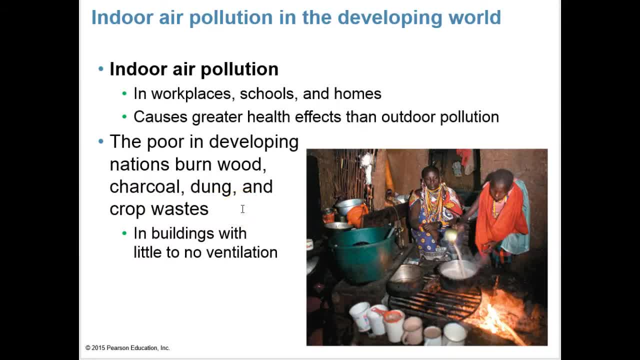 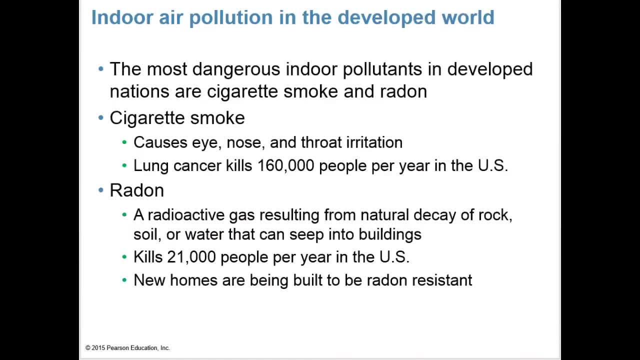 and dung and crop wastes, and then this is occurring in buildings with little or no ventilation. The most dangerous indoor pollutants in developed nations are cigarette smoke and radon. Cigarette smoke causes eye, nose and throat irritation and eventually can lead to lung cancer. 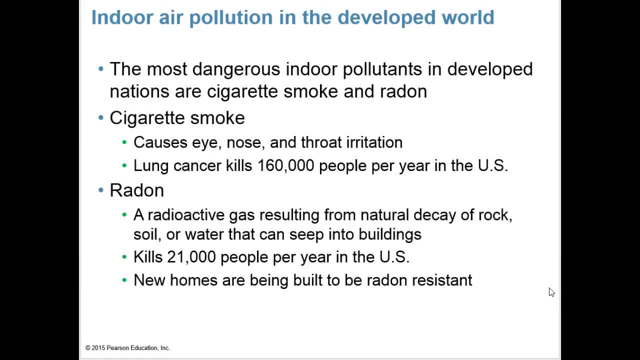 which kills 160,000 people per year in the US. Radon is a radioactive gas resulting from the natural decay of rock, soil and water. It kills an estimated 21,000 people per year in the US. New homes are built to be radon-resistant. 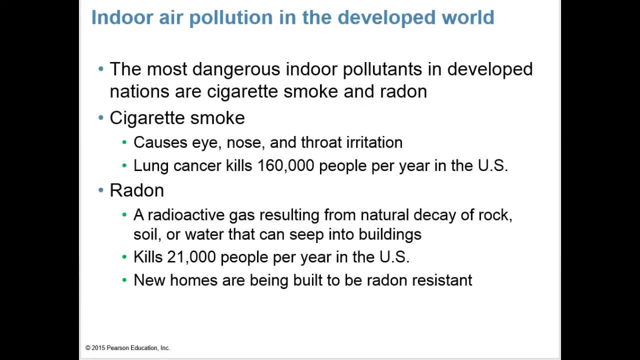 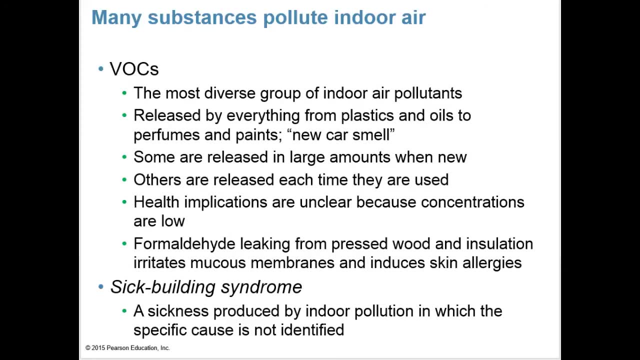 but not all older homes are and not all people are aware of the problem. Volatile organic compounds, or VOCs, can make up the most diverse group of indoor air pollutants. They're released by the air and they're released by the air. 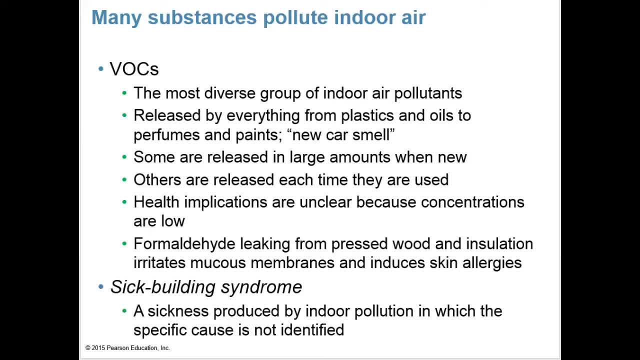 They're released by air pollutants. They're released by everything from plastics and oils to perfumes and paints. They even give us that new car smell. Some are released in large amounts when they're new, when the products are newer. Others are released each time they're used.